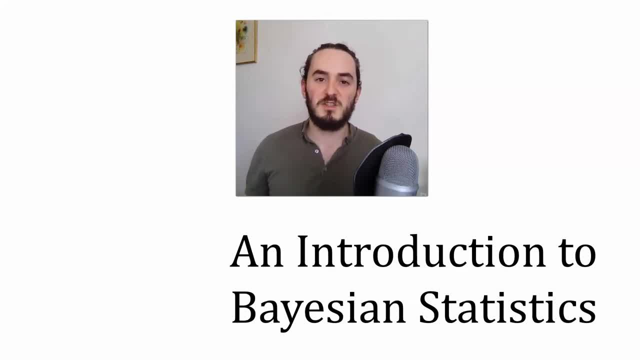 to know more about probability theory, or if you're interested in using this professionally as a data scientist or a programmer. We're going to begin by asking some pretty profound questions, like what probability even means. We'll think about it in the context of simple events like 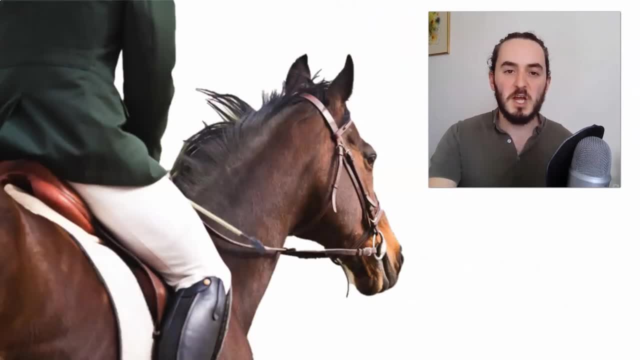 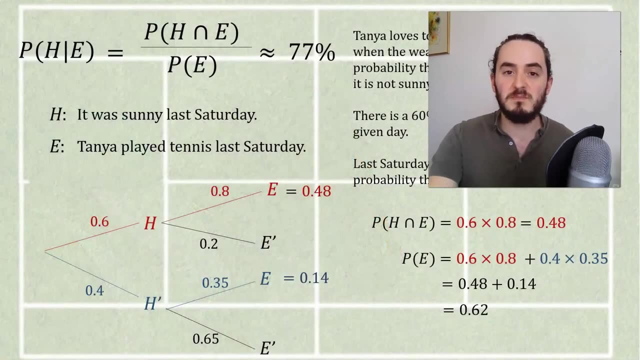 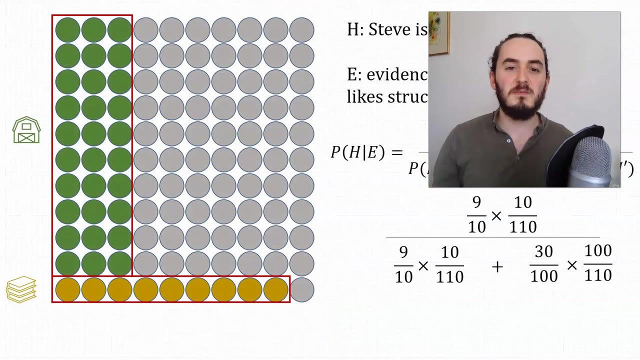 dice rolls, but also one-off events like horse races. We'll then look at conditional probability and how it can help us solve some pretty unintuitive problems. We'll use things like tree diagrams and also consider distributions like the normal distribution. We then tackle Bayes' theorem head-on, trying to keep things as visual, colourful and intuitive as possible. 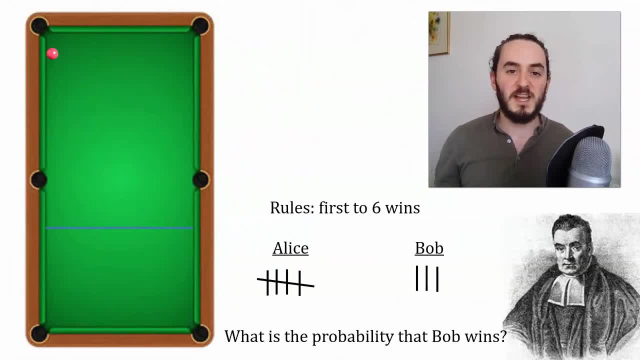 throughout. Finally, we have a look at the puzzle that kicked off this whole thing 250 years ago, when Thomas Bayes proposed a puzzle involving a billiards table. I really hope you enjoy this course and it helps you understand Bayesian probability deeply and intuitively, and that it helps you understand the world a little bit better. Hello and welcome to. 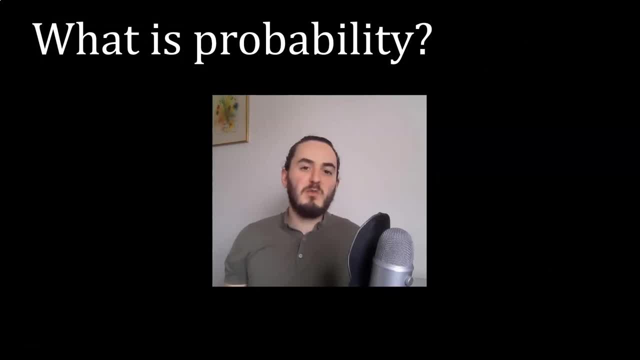 this first lesson on Bayesian statistics, We're beginning with what might seem like an obvious question: What is probability? Now, it's worth remembering that probability is actually a relatively new area in mathematics. It's a relatively new area in mathematics. It's a 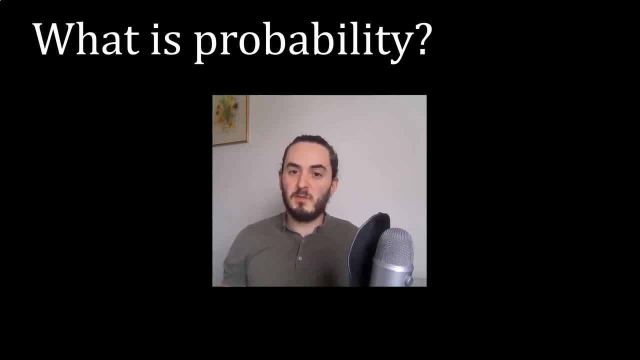 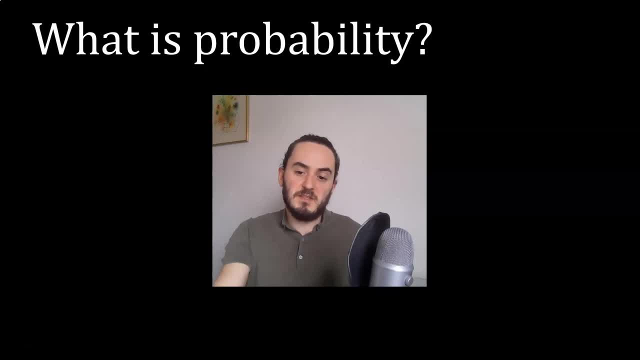 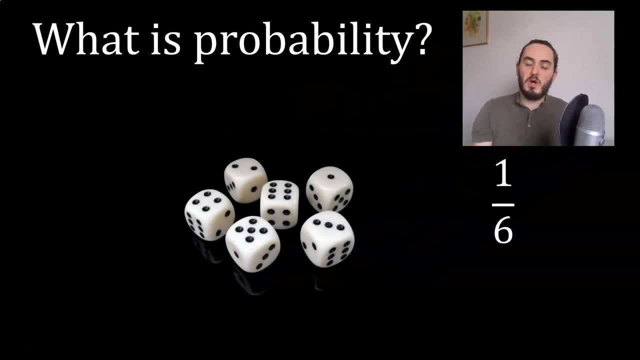 lesson is establish how we can make sense of what it means, for example, to say the probability of, say, rolling a dice and rolling a six is one in six. So we're going to think about two different ways that you might characterise this, and only one of them is really going to be compatible. 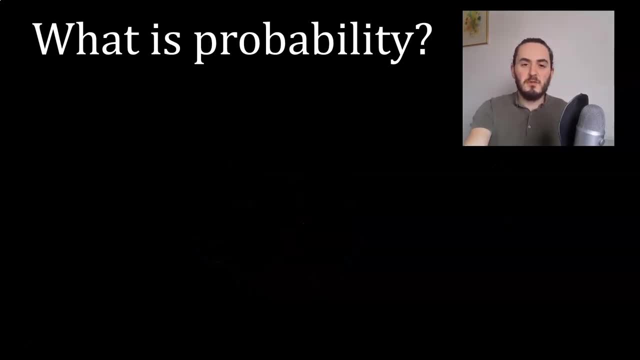 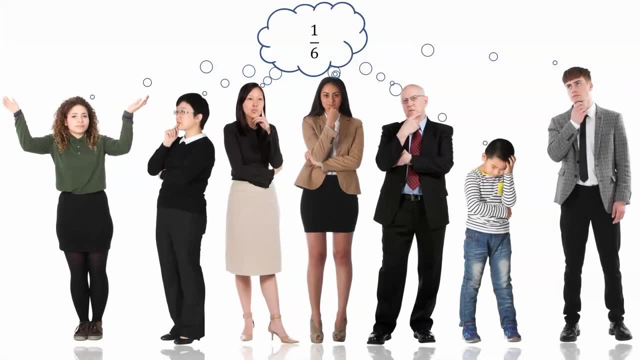 with what we want to achieve in this course. So the first way we could think about this is from an objective standpoint. So why, for example, do we say that the probability of rolling a six on a dice is one sixth? Well, one way to characterise this is that we all think it's. 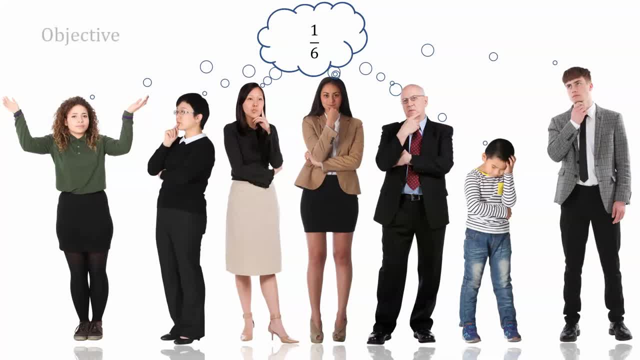 one sixth on a fair dice, And that's because this reflects some objective reality. Now, one way to cash this out is from a frequentist standpoint. Let me explain what that means. Let's say we're considering dice. You might roll the dice once, twice, three times, four times, five times, six times. 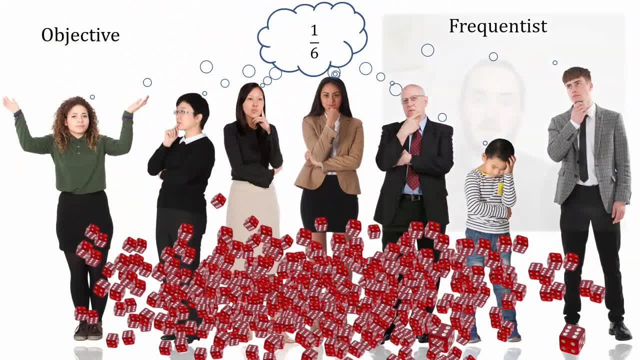 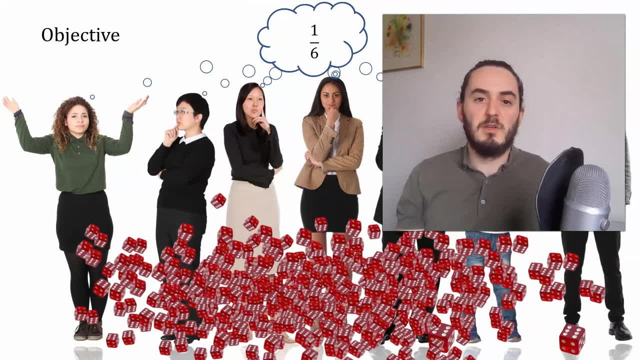 twice, a million times, maybe even an infinite number of times. What you can then do is you could take a random sample, maybe even an infinite sample, from those rolls and you could say what proportion of those did a six land face up? And we know that, as the number of rolls tends to. 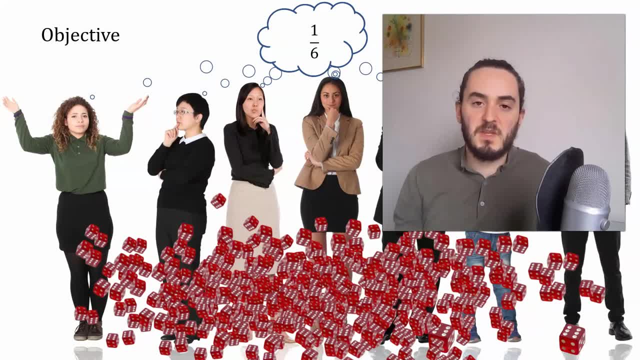 infinity, the proportion is going to tend towards one sixth. So one way to explain what the probability is is in terms of frequencies. We would say: if the event was to happen infinitely many times, what would the proportion be of the thing we're interested in? 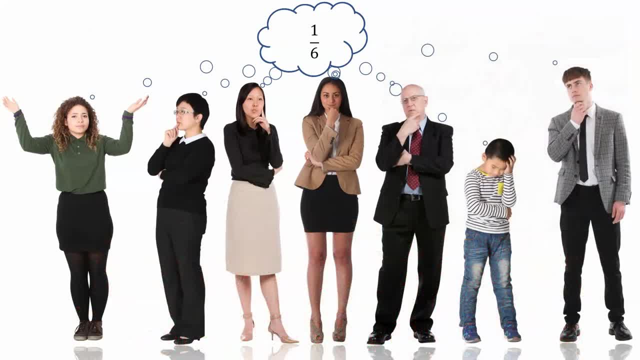 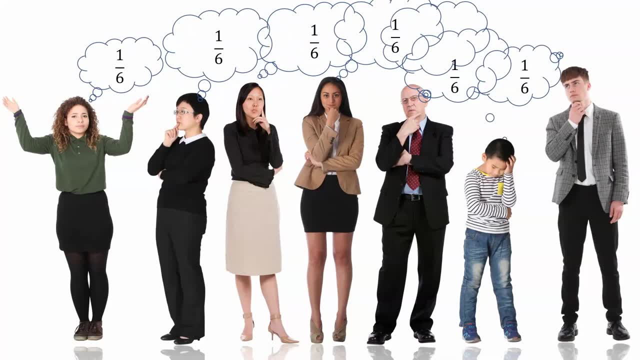 Okay. so what could be a different point of view? Well, a different way to think about it is a subjective approach, which is to say that each person has their own reasons for believing a certain probability. So this subjective stance is the one that's going to form the foundation. 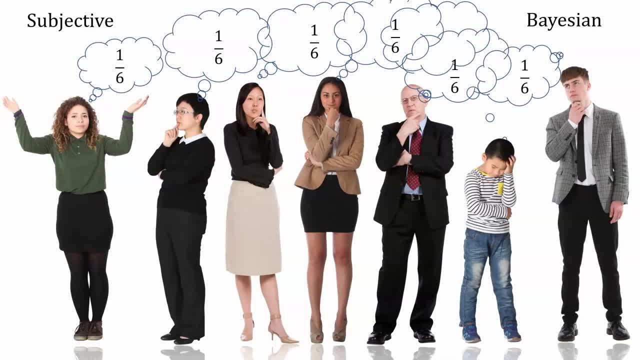 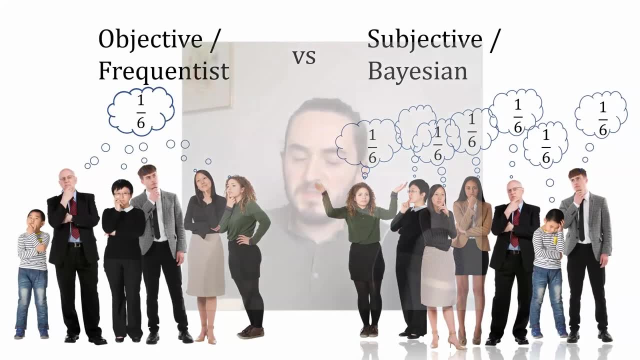 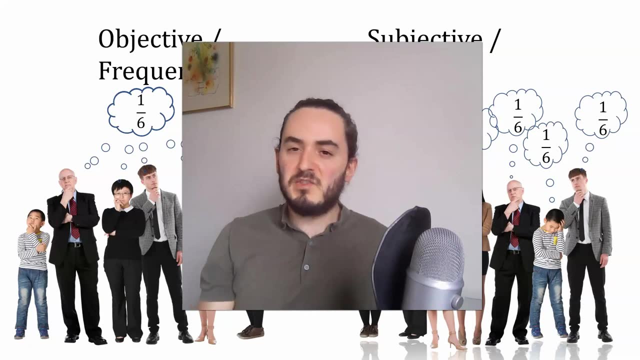 for what's going to become our Bayesian model. Which is it then? Is it the subjective Bayesians or is it the objective frequentists? I think a lot of people's intuition at first is to say that the subjective one seems a little bit. 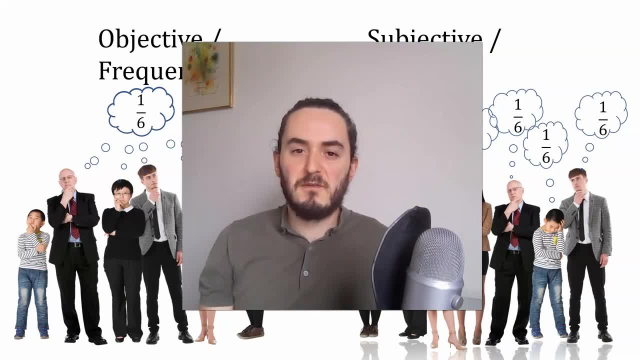 too wishy-washy, a little bit not set in stone enough. So, as you can probably guess, since you've signed up to do a course in Bayesian statistics, I think there are some very good reasons for taking a subjective Bayesian model. It's not subjective in the sense that you can think whatever. 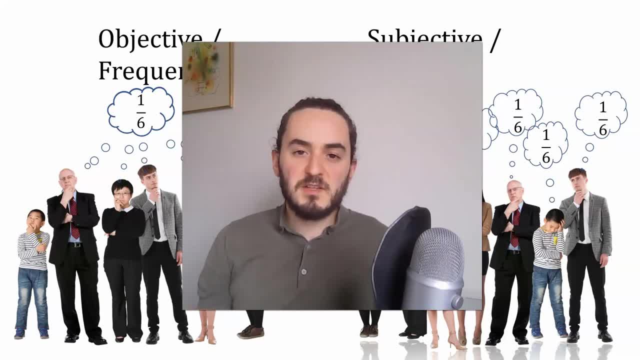 you want. but it's not subjective in the sense that you can think whatever you want and you can think whatever you want, but it's subjective in the sense that each person might have a different answer to the question. Now I'm going to give you two reasons for thinking this One is to attack. 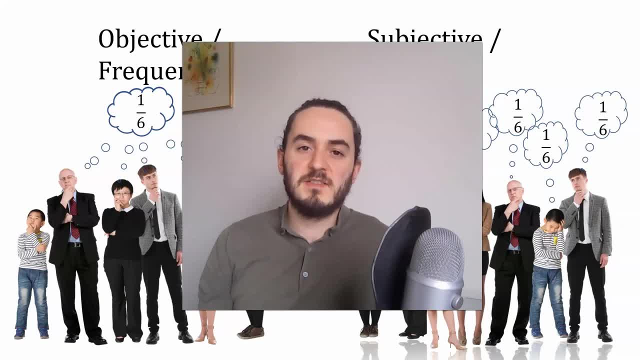 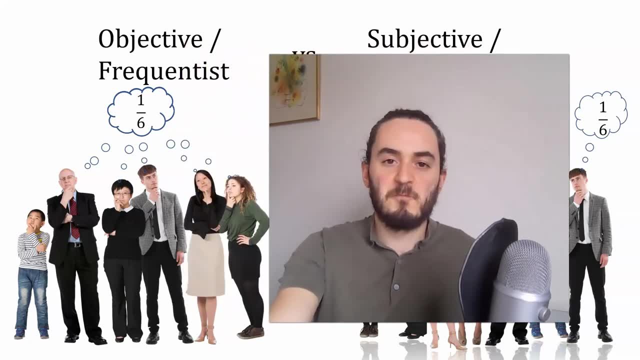 the frequentist position, show that it doesn't work in all cases, and then in a different situation. I'm going to show you a great reason for thinking the Bayesian subjective model is actually really good. So this frequentist model is perfectly good. when we're thinking about dice, No problem. 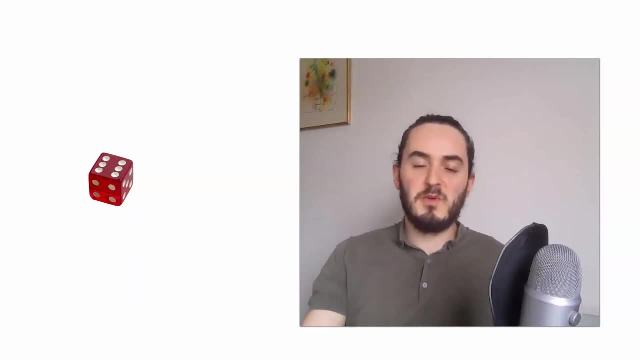 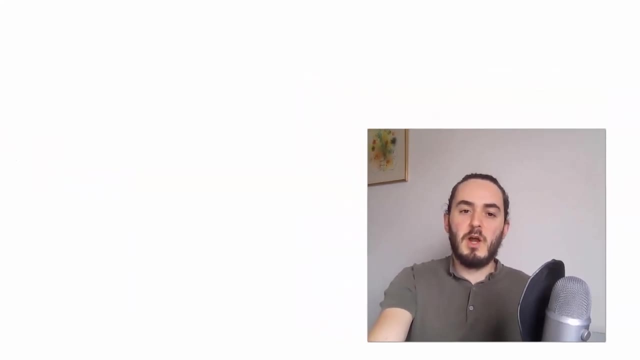 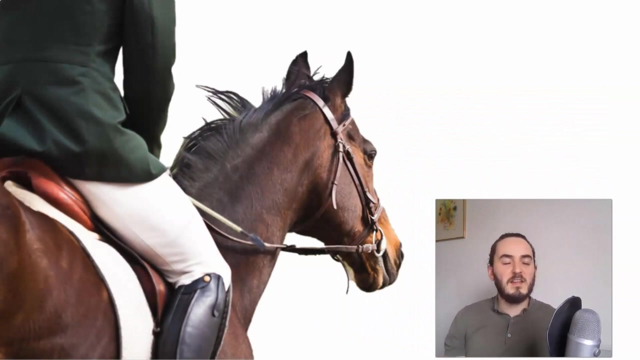 we could imagine wrongly the dice many times. We could at least hypothesize wrong infinitely many times. But what about when we've got a specific one-off event? Take, for example, a horse race. Let's say it's the Grand National and here's our horse. and, if you'll excuse the pun, let's say his name is Bayes Camp. 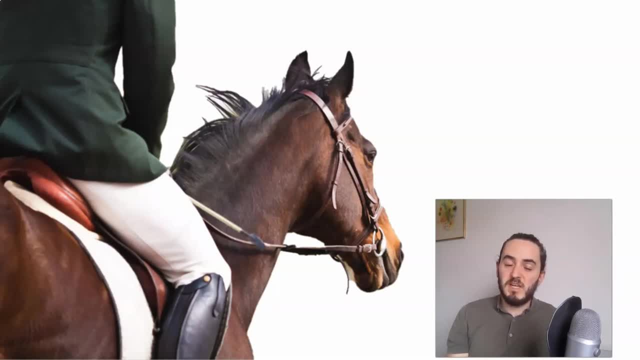 So what's the probability that Bayes Camp is going to win? It's the sort of thing that anyone who's going to bet on the horse race wants to know. It's the sort of thing that's going to win. It's the sort of thing that statisticians want to know. Now, there are some pretty good reasons. 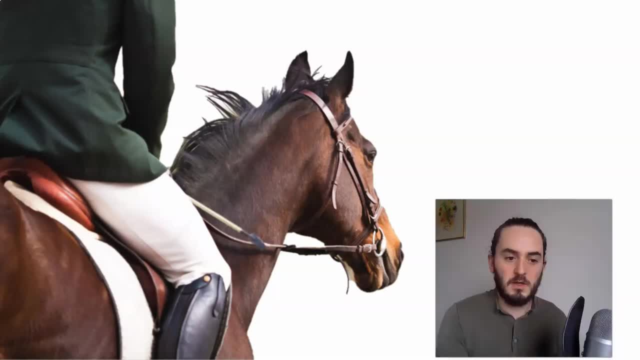 for thinking that frequentist account doesn't really work here. So here's what the frequentist is going to have to say about this horse race. We're going to have to hypothesize an infinite set of horse races, So we're going to have to imagine this single horse race happening. 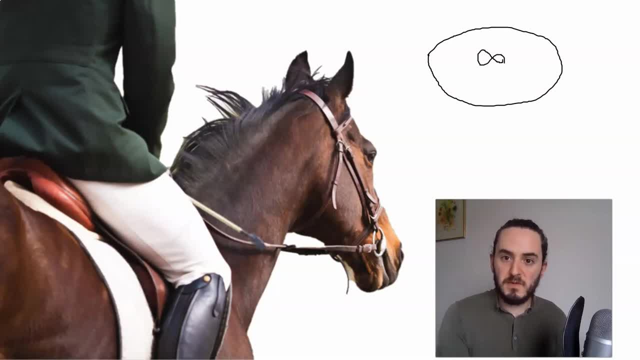 infinitely many times. Now, from this, we're going to have to draw out a random sample of these horse races, So we're going to have to hypothesize an infinite set of horse races, Just like we might consider a random sample of dice being thrown, And maybe this sample is infinite. 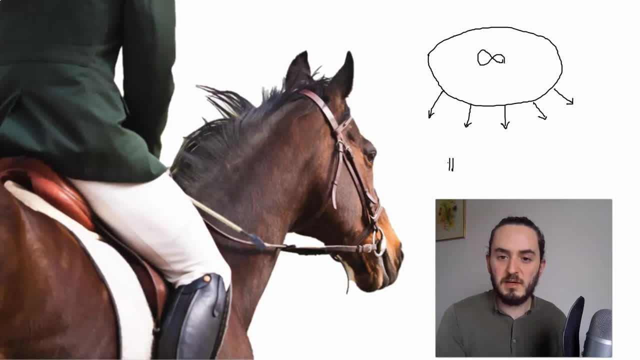 And then what we're going to do with this is we're going to count how many times did Bayes Camp win And we're going to divide that by how many races there were, And whatever number that is. that's going to tell us the probability that Bayes Camp will win. 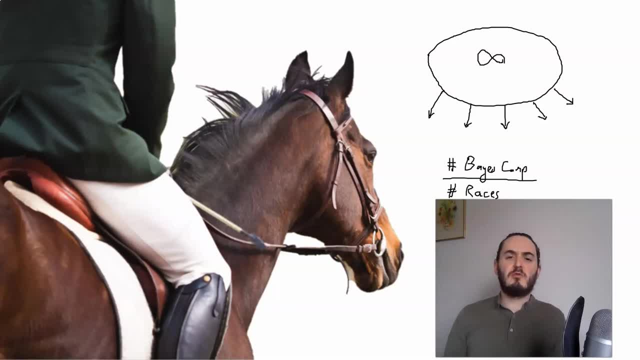 the Grand National. Now, a lot of people think there's quite a lot wrong with this model, for two reasons. The first is: what does it even mean to imagine an infinite set of a single event like the Grand National happening? It's not something that can happen more than once. It's. 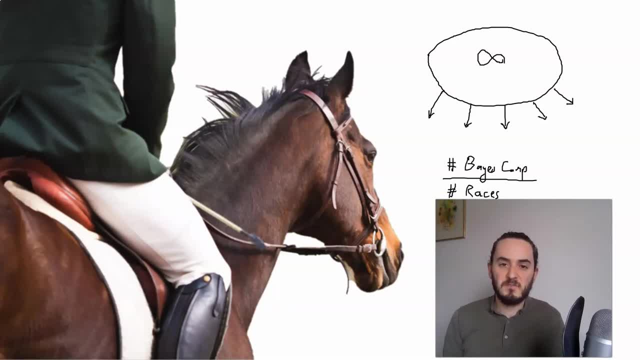 pure imagination to speculate all of these races. And then what does it even mean to draw a random sample from a hypothetical set? So it seems like there are some pretty good reasons for thinking that the frequentist model is no good in situations that are just one-off events. 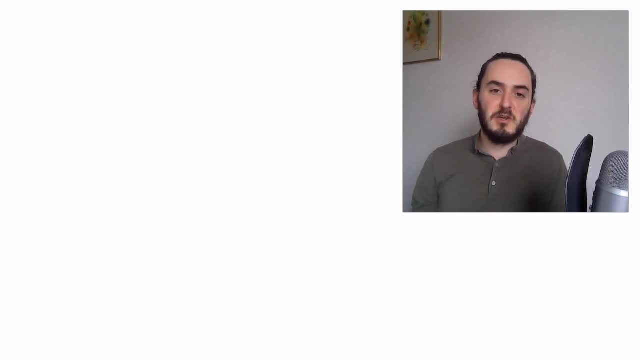 But let's look at some reasons why the Bayesian model might actually be really good. So suppose I told you that my partner was expecting a baby and we didn't know if it was going to be a boy or a girl. And just for the sake of simplicity here we're going to ignore some biology and assume. 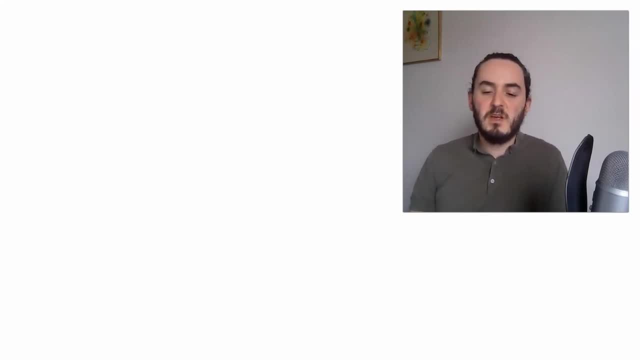 that everyone is either male or female. So what can we say? Well, here's Alan, and he's my uncle. Now Alan thinks that the probability that the child will be male is 50%. Now he has no reason to think. it should be male, should be female. so he's going with 50%. So that seems a pretty. 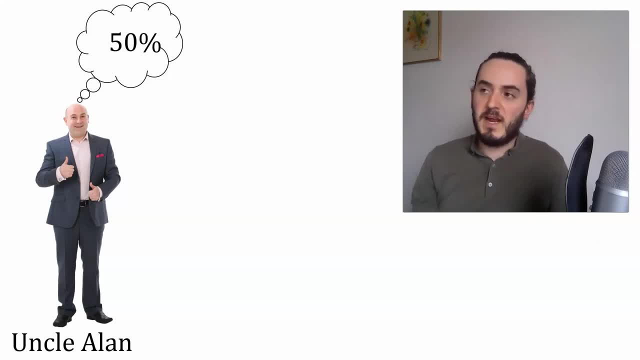 reasonable thing for him to say. Would we say that this probability is correct? I think a lot of people would. Now here's our friend Anna. Now Anna is a doctor and Anna has just written an article for the World Health Organization showing that in my area, 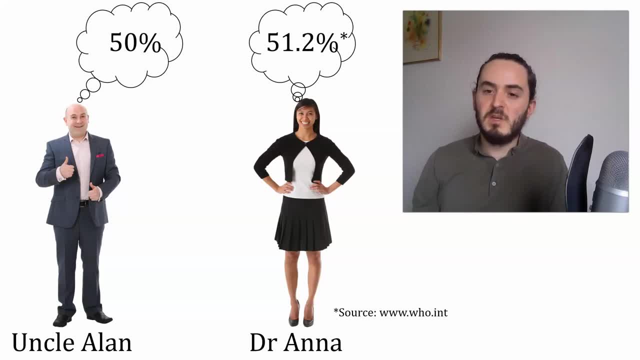 51.2% of all children born are male. So is Anna's view more correct than Alan? She certainly has more information, but is it fair to say that she's right and he's wrong? It would be unfair, I think, on Alan to say this. Anna has more information and no doubt if Alan. 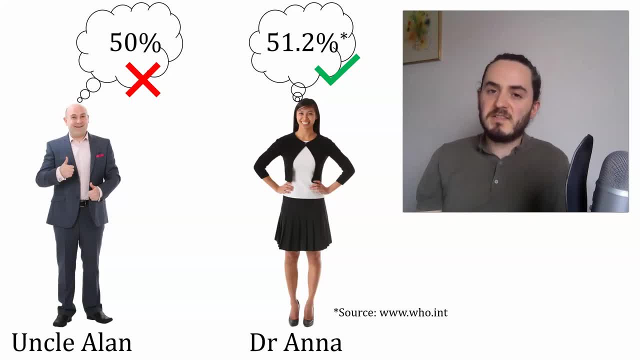 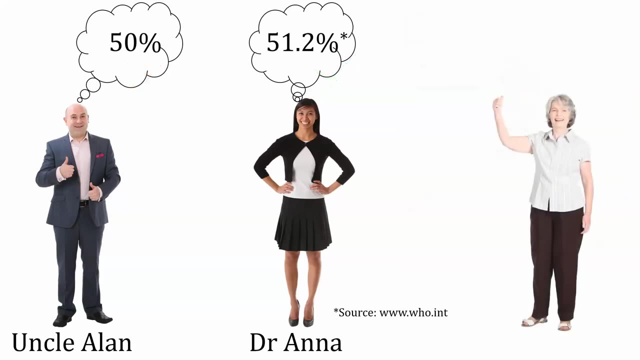 read her article, he might change his mind. But as things stand, it would be irrational for Alan to say 51.2%, because he has no reason. Now let's throw another character into the mix. Here is Sarah. Now Sarah is our midwife. 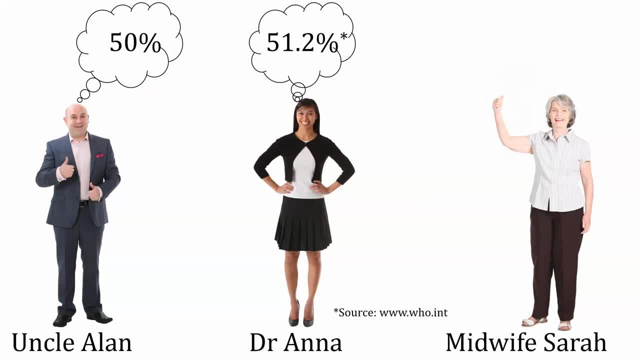 and Sarah has just performed a scan. Now the scan isn't 100% accurate, but it looks to her like it's male. She thinks the probability the child is male is 95%. So what do we say now? Is it right to say that Sarah's probability is correct? 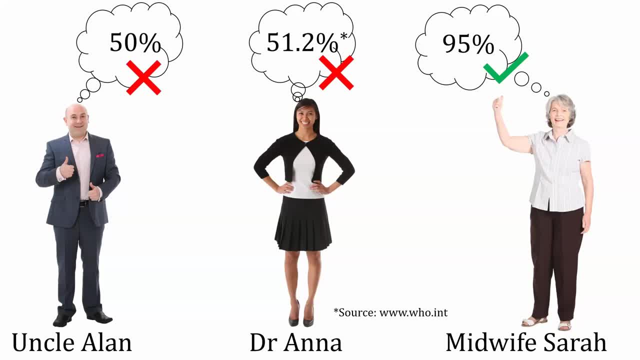 And Anna and Alan's is incorrect. Most people's intuition is that this is not the right thing to say. Sarah certainly has more information, but if Alan was to suddenly say no, I think it's 95% likely the child will be male. without that information, that would be irrational. 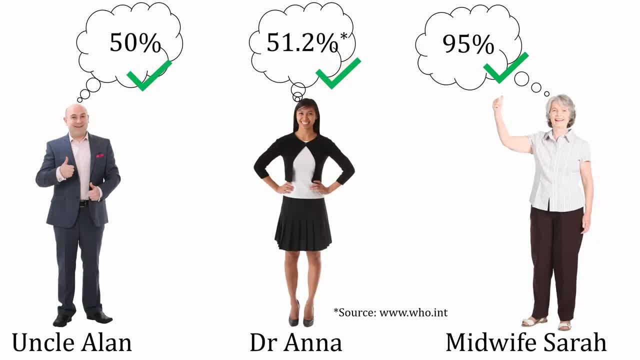 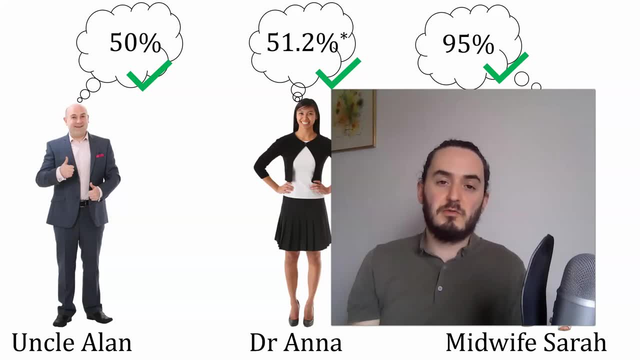 So the Bayesian approach is to say that actually all three might be correct And really the probabilities represent each individual's degree of information. So the Bayesian approach is to say that actually all three might be correct And really the probabilities represent each individual's degree of information. 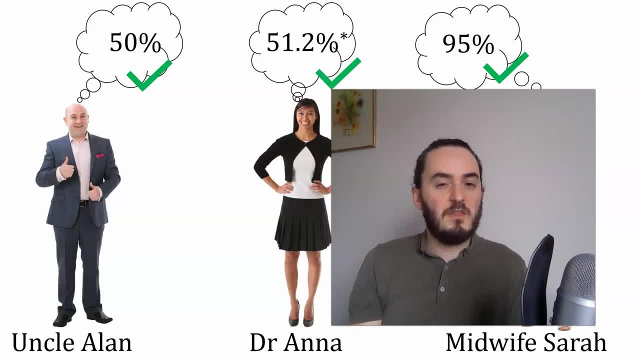 in which probability is subjective. it's not that you can think whatever you want. So Sarah can't look at her scan and say she still thinks it's 50%. that would be irrational. Alan can't, in the absence of any other evidence, say he thinks it's 95% likely to be male. that would be irrational as well. 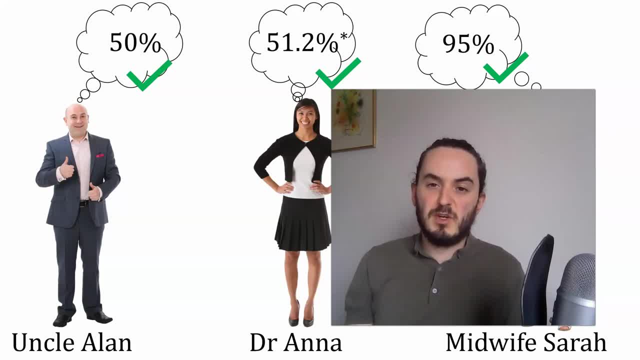 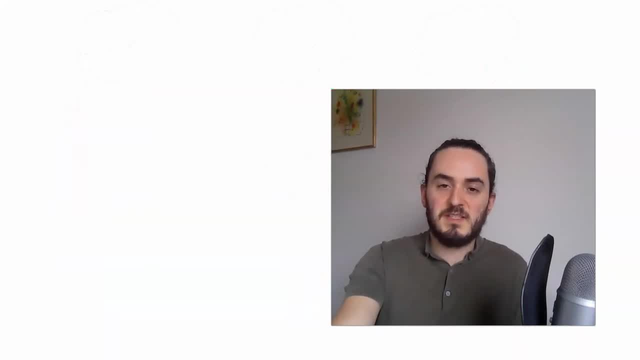 Each person has a certain amount of evidence which forms their degree of belief or the measure. Each person has a certain amount of evidence which forms their degree of belief or the measure of their uncertainty. uncertainty, So that's the Bayesian approach to this. So degrees of belief are going to form. 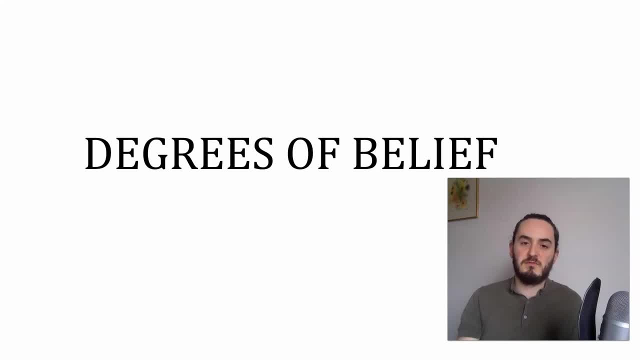 the underpinning of everything that we're looking at in this course. I hope you found that first lesson interesting and I hope it gave you a framework with which to think about probability for the rest of the course. See you in the next lesson. We're now going to look at conditional. 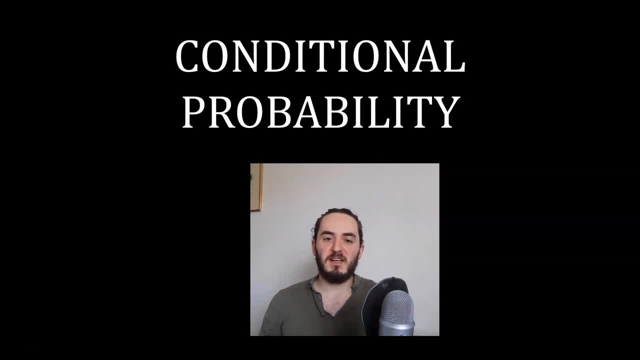 probability. and we're going to begin this by looking at a really simple example, but one that helps build some intuitions which will help us build up to looking at Bayes theorem in full later on in the course. So let's start with a super simple and kind of silly case. So we've got these. 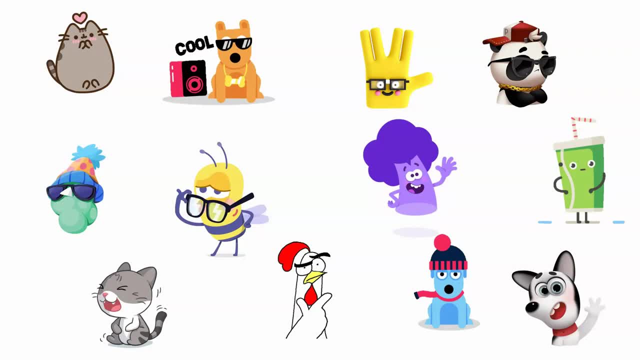 12 characters here and there are loads of different probability questions we could ask if we were thinking about randomly selecting one of them. So we could categorize these guys in loads of different ways, but one way we could do it is according to whether they're a dog and 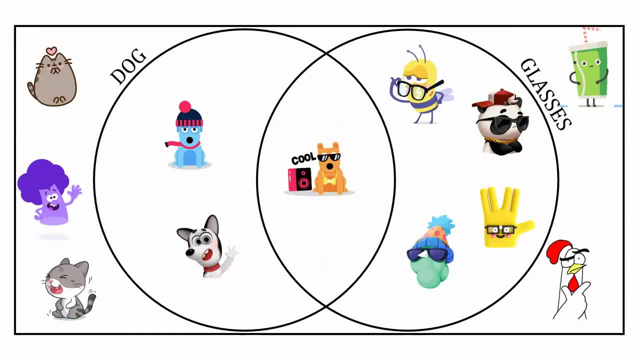 whether they wear glasses. So that guy in the middle is the only one who is both both a dog and wears glasses, And we've got some dogs who don't wear glasses and some non-dogs who do wear glasses, and so on. Now that we've got this visualized, 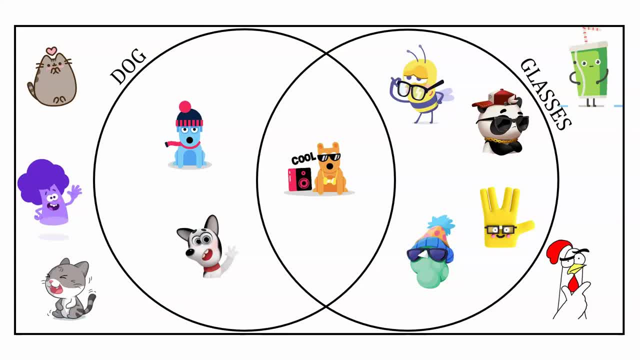 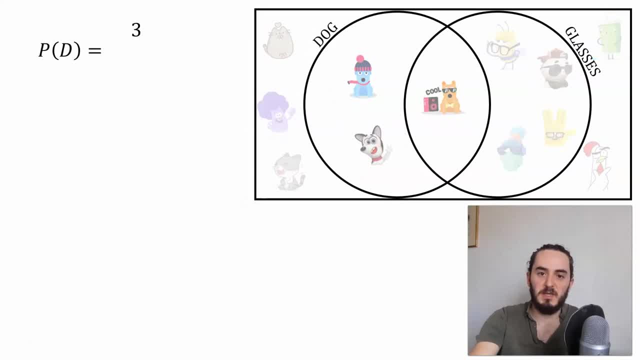 we can ask some probability questions about it, ranging from the really really simple, such as: what's the probability that a randomly selected character is a dog? and there's no tricks here, it really is, just there are three dogs out of 12 characters. 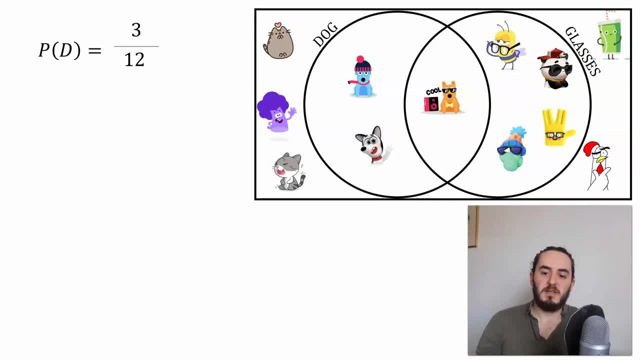 so three out of 12, to a slightly more complex question such as: what is the probability that a randomly selected character is a dog, given that they wear glasses? now, for this we need to think about conditionality. so the condition here is that the character is wearing glasses, which means we're going to restrict ourselves to only thinking about 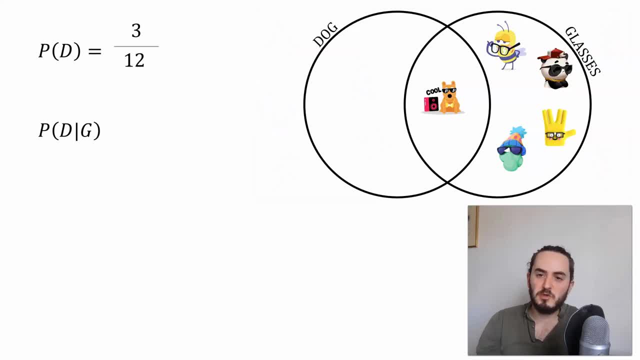 these five guys who wear glasses, so as of zooming in on that, ignoring everything else. so, given that they wear glasses means we are looking at a probability out of five, so there are only five characters who wear glasses, and the question is how many of them are dogs? and the answer is of 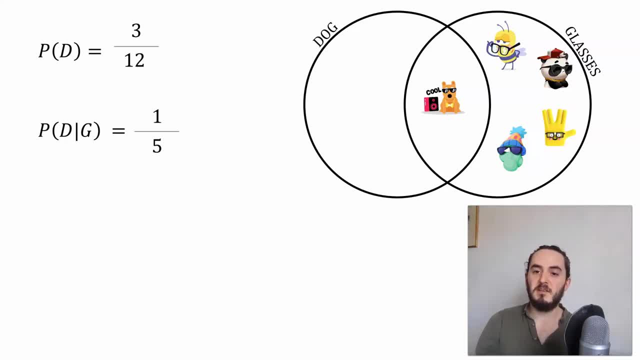 course one. so one out of five is the probability that a character is a dog, given that they wear glasses. okay, so far, so simple. um, how could we formalize what we've just done and make a general rule about it? well, in this example, we're just counting and really. 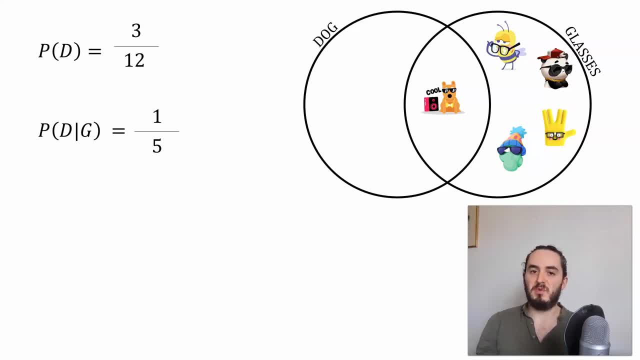 we want our rule to relate to probabilities and that's what we're going to practice, actually, in the next video. but for now we can say that the one guy in the middle, that guy who represents being a dog and wearing glasses, that region is the can represent the probability of a character being 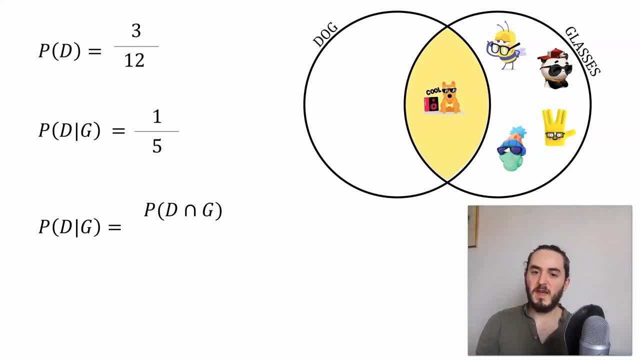 a dog and wearing glasses, so that region there can represent that probability. so that's the probability of dog and glasses. now the whole, uh, the whole region is obviously the probability of a character wearing glasses. um, since it was, that was what was the condition, so formalized in this way, we've now got it wrapped. 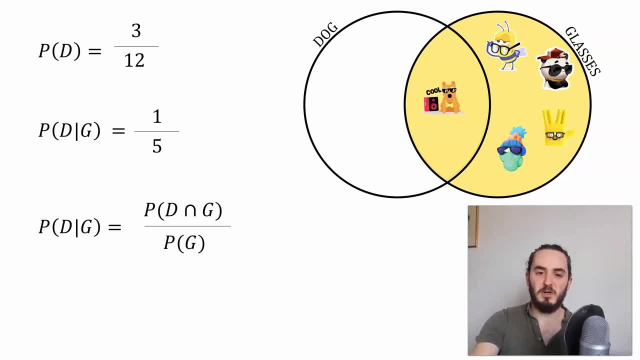 up in terms of probabilities, which is going to be useful for us later on. now i'll call this for now baby bayes theorem. it's most of the way to formulating the full bayes theorem, but it's not quite there yet. but it's really useful. we can already solve some pretty complicated stuff with. 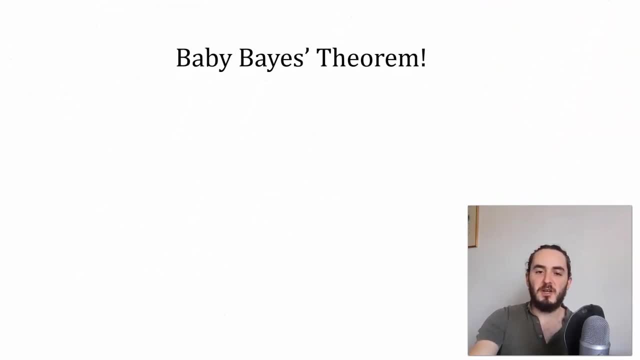 it. um, just a little note on the letters that we use. typically i'll be using h and e rather than, you know, dog and glasses, and d and g, and the reason for that is that, um, we're often thinking about the probability that a hypothesis is true given some evidence. so, in general, we're going to 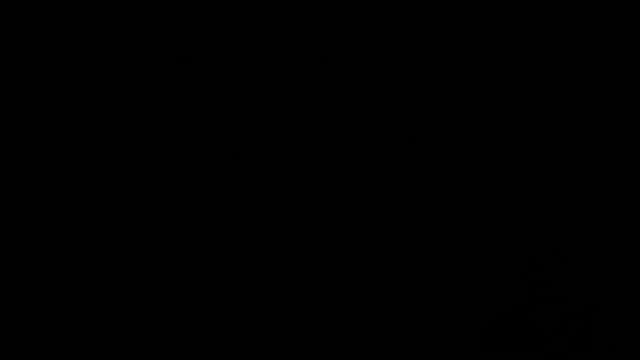 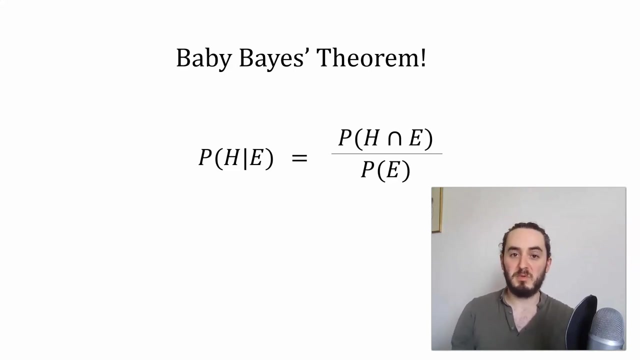 be using h's and e's in most cases. so now that we've derived this baby bayes theorem, let's apply it directly to an example of a baby bayes theorem. let's apply it directly to an example of a baby bayes theorem that uses probabilities and not just counting. it's a pretty simple example and i do. 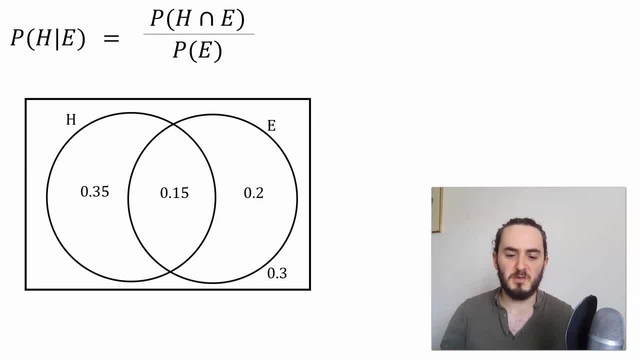 encourage you to pause the video and try to solve it yourself, just to check you understand what's going on here. all right, so in order to work this out, we're trying to work out the probability of h given e. so it's often easiest to begin in these cases with the probability of of e. so what's been? 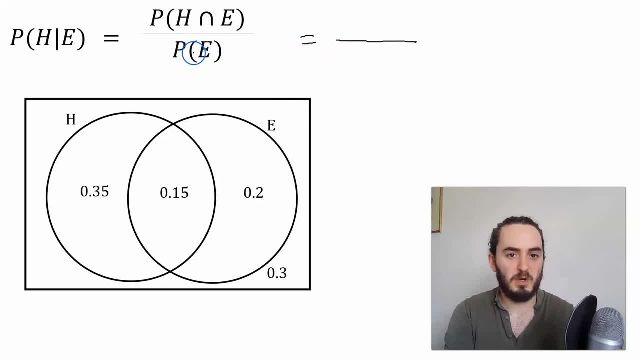 given. so, um, what is the probability of e? well, it's not just 0.2, it's the entire bubble, so it's everything included in it. so 0.2 plus 0.15, so we've got 0.35 here, and the probability of h and e, well that's. 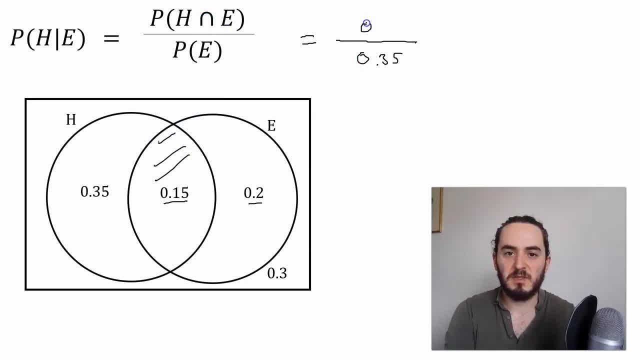 just this intersection here. so that's 0.15. so that's our answer and you can do this in your head if you want, or you can use a calculator, but it's. it's a pretty simple example of what's the probability of h given e when we've got the information presented to us. 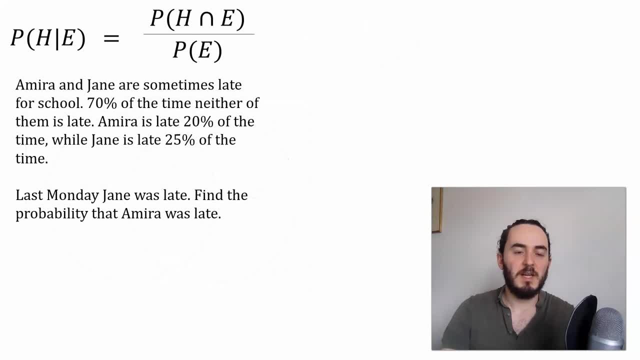 as probabilities in a venn diagram. now let's take a look at a much harder example here. so in this one, the challenge at the beginning is to actually just visualize this, which will involve drawing a venn diagram for ourselves. so here's the question. amira and jane are sometimes late. 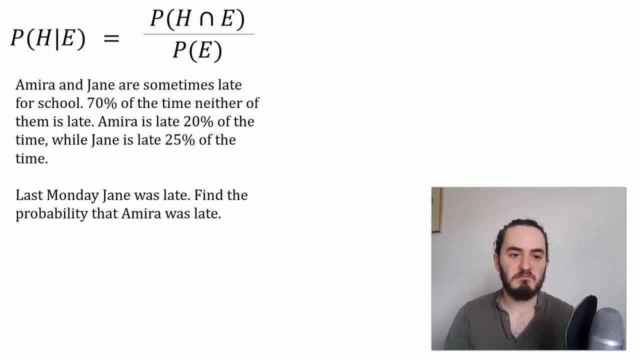 for school seventy percent of the time. neither of them is late. amira is late twenty percent of the time, while jane is late twenty five percent of the time. last monday jane was late. find the probability that amira was late all right. so, uh, the first thing to do is just give a bit of terminology or use a bit of terminology. 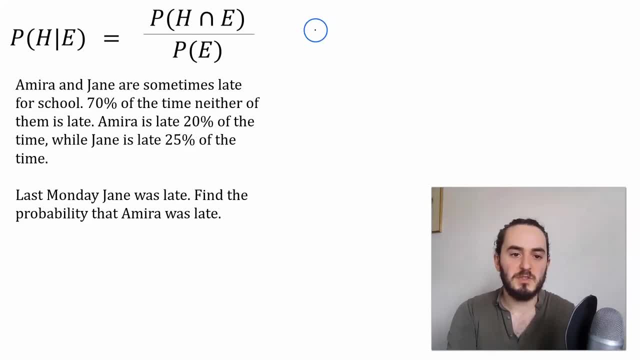 to formalize what's what we've actually been told. so okay, what's our evidence here? well, our evidence is that last monday, jane was late. twenty five percent of the time jane was late, twenty five percent of the time was late. so let's say that um e for us is the represents jane, jane being late, so jane is late. 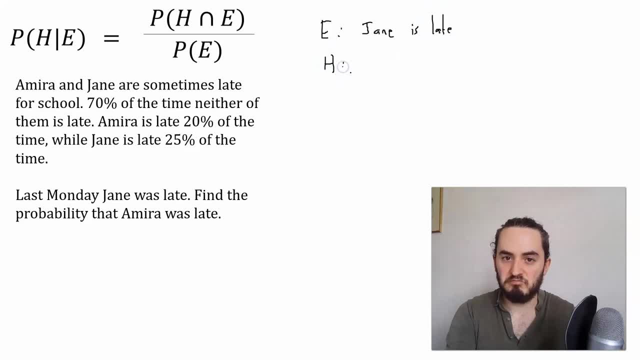 and our hypothesis. the thing that we are interested in testing is whether amira is late. so h is going to be amira is late. all right, let's now try to write down uh, using this note, but also to determine if jane is late or not. so let's go to our professor, do 안�i's professor. 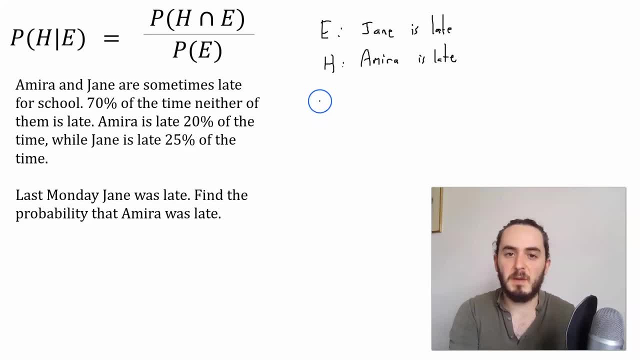 noth and then we write down some of the information that we've been given. so 70 percent of the time, neither of them is late. so there are actually different ways to write down that something hasn't happened. you'll often see, for example, if we wanted to write that jane isn't 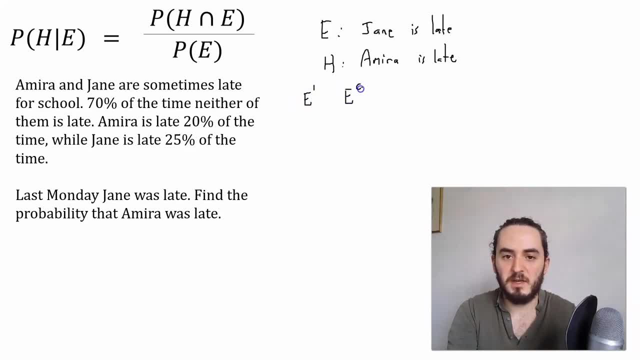 late. you'll sometimes see it written as e prime or e dash like that. you'll sometimes see it written as ec, that stands for the complement. you'll sometimes see a hook: e like this, that's okay, E like this. I'm going to use this one, the E dash. So what we've been told is the probability. 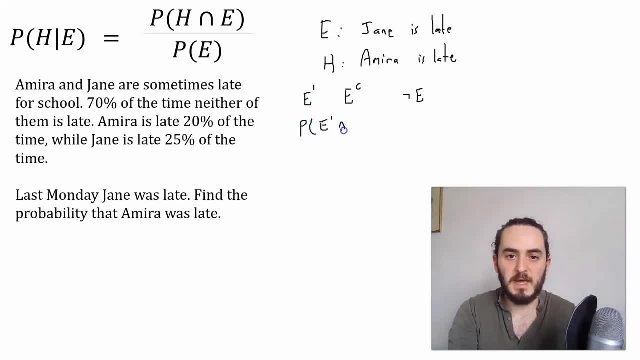 that Jane isn't late, so E dash and Amira isn't late, so that's H dash is 0.7.. And we've also been told that the probability that Amira is late, so that's the probability of H, is 20%. 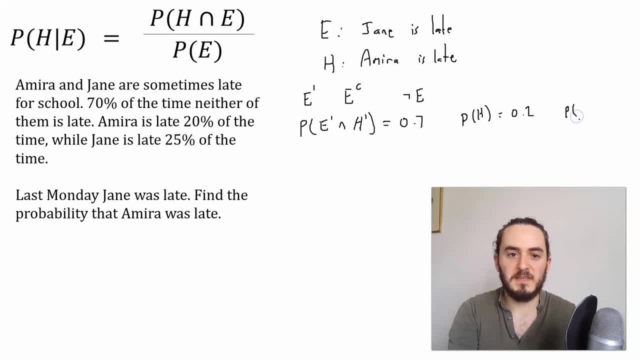 so that's 0.2.. And we've been told that the probability that Jane is late, so the probability of E, is 0.25.. Now can we represent this all on a Venn diagram? So really this is the main. 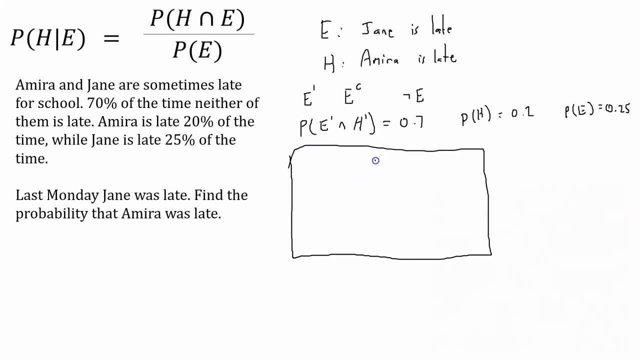 challenge. So this bubble here can represent H, so that's Amira being late, and this bubble here can represent E, so that's our evidence and that's Jane being late. Now the first thing we can do is put a 0.7 on the outside. 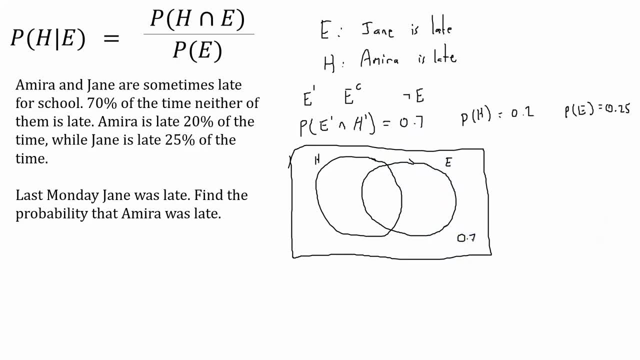 Because that's the condition that neither of them are late. Next, what can we say? Well, I know that the entirety of this H bubble is 0.2, because the probability that Amira is late is 0.2. So this entire bubble here has got to sum to 0.2.. So if all of this bubble 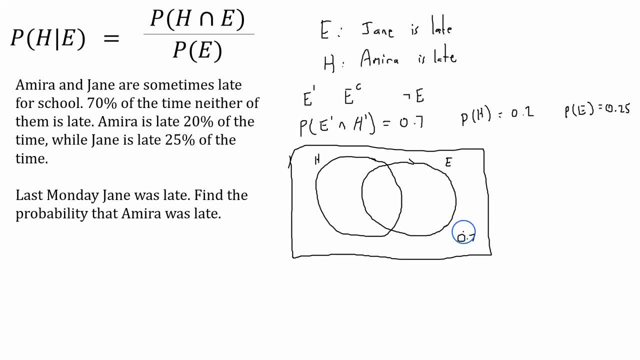 sums to 0.2, and we've got 0.7 here. the only part unaccounted for is this section here. Now, if I've got 0.2 here, let's just keep track of this and 0.7 on the outside. 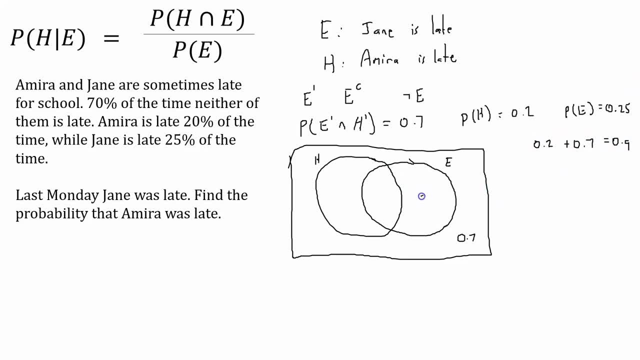 that takes us to 0.9.. So the only unaccounted for region is this, and it's got to be 0.1, because all of the probabilities need to sum to 1.. Well, I now can work out the rest quite. 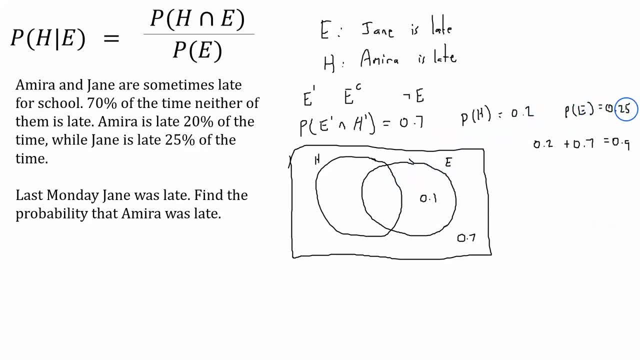 easily, because I know the probability of E is 0.25.. Now I've got 0.1 here and I've got 0.2 here and I've got 0.2 here. So there is 0.15 remaining And I know that probability. 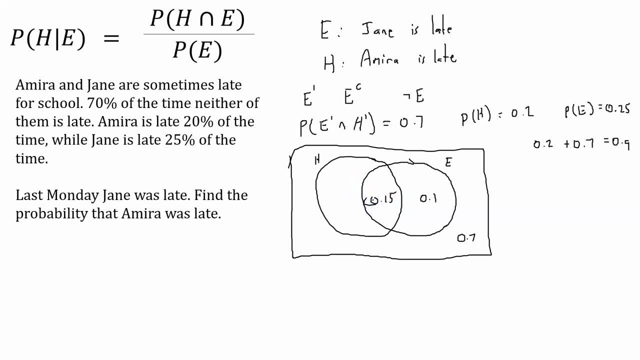 of H is 0.2,. now I've got 0.15 here, and so 0.05 remains. Okay, so there's our picture. We've got the information represented in the Venn diagram. We're now in a position to actually go for the main question. So what is the probability? 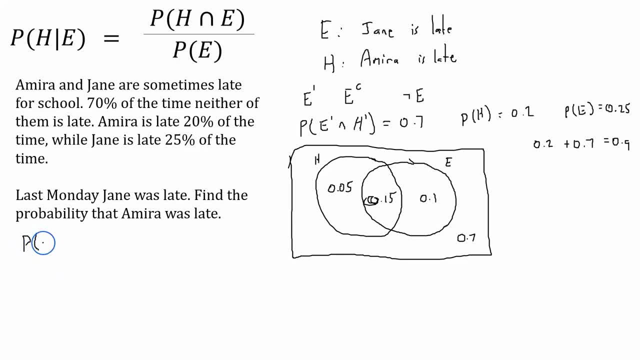 that um a mirror is late H, given the information that Jane was late, given our evidence that Jane was late, Well, using our baby Bayes theorem, it's the probability, it's the intersection. so that's the probability that they are both late, which we now know is 0.15, divided by 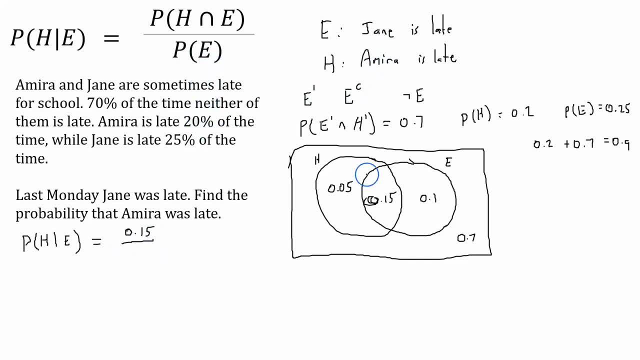 the probability of E divided by our evidence. So that's the probability that Jane is late, and that's all of this here. so that's 0.25.. Okay, so that's 0.25.. 0.25.. And that's going to simplify down to three-fifths, or alternatively, 60%. So we 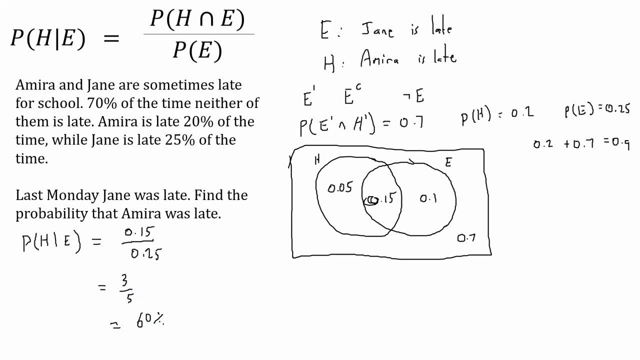 now know that, um, when Jane is late, a mirror has a 60% chance of being late. So most of the time she's late- 20%, or rather, in general her probability of being late is 20%. but 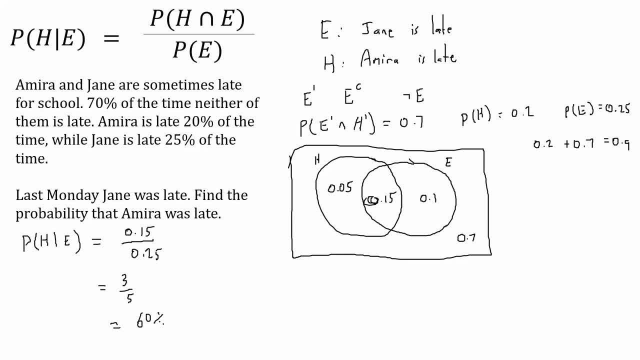 if Jane is late, there is a 60% chance of being late. So we now know that, um, when Jane is late, there is a 60% chance that a mirror will be late as well. So one way to think about that is that Jane being late. if we learn that. 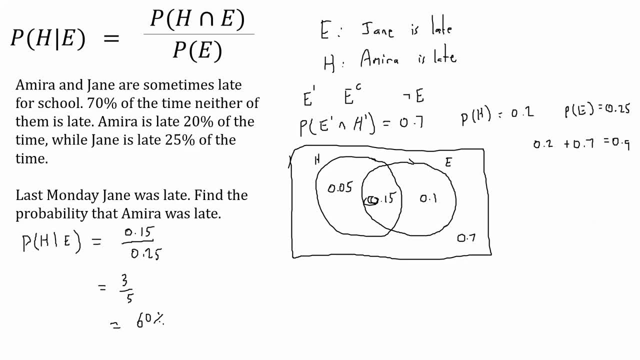 Jane is late, we update our idea about what the probability that a mirror is late. In fact, Jane being late seems to make a mirror more likely to be late, And it's that kind of thinking which is going to help us sort out Bayes theorem later on this idea of updating. 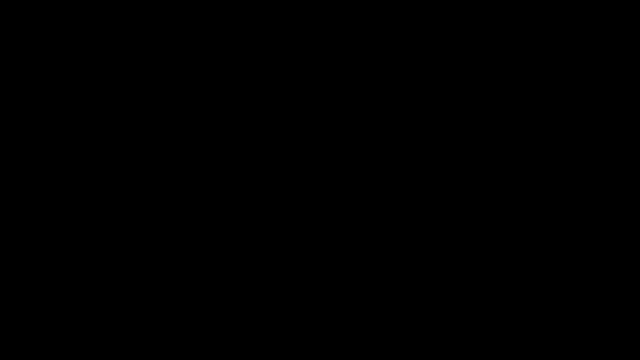 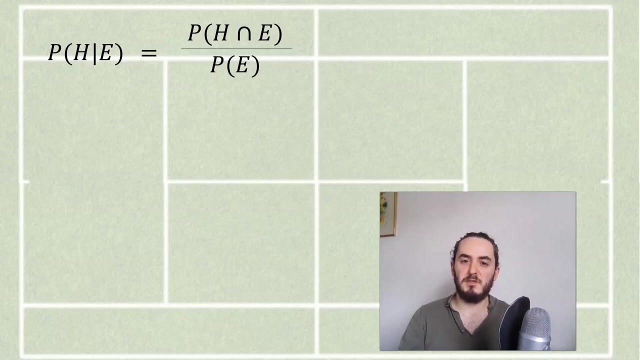 our probability given some new evidence. Let's now have a look at an example where we apply our theorem to examples that can't easily be solved using simple Venn diagrams. So here's a question. Tanya loves to play tennis, but especially so when the weather. 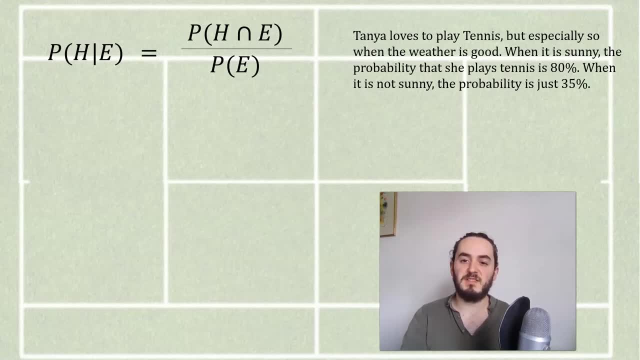 is good. When it is sunny, the probability that she plays tennis is 80%. When it is not sunny, the probability is just 35%. There is a 60% chance that it is sunny on any given day. Last Saturday she played tennis. What is the probability that it was sunny last? 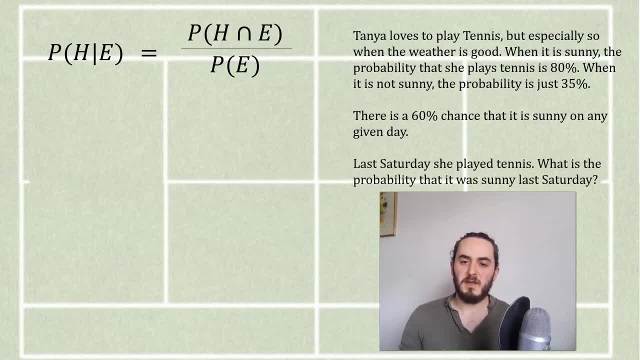 Saturday, Okay, so obviously we think that there is a 60% chance that it is sunny on any given day normally, But we've got some new evidence, which is that she played tennis And that's going to be relevant and could lead us to update our opinion of what the probability. 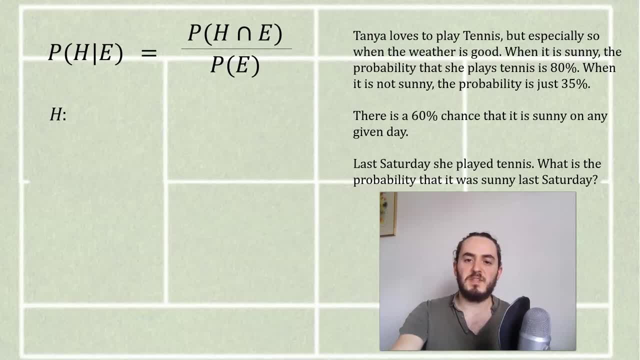 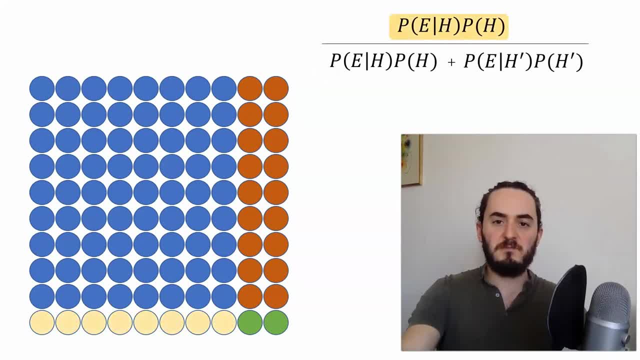 crystal clear about where each bit comes from This numerator. well, that represents these yellow guys down here. So they're the ones who have the disease and who they've been told that they have it. So it's the probability of the evidence. given the hypothesis, That's the probability of having a 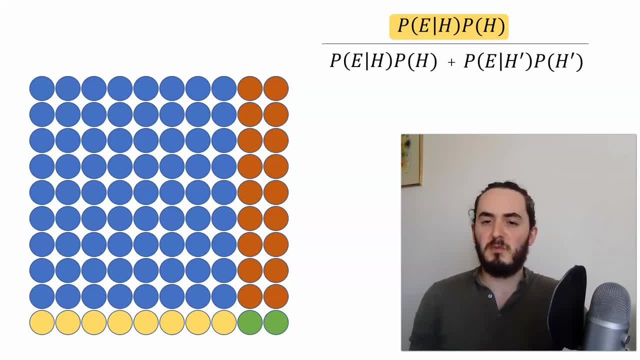 positive test result, given that you have the disease multiplied by the probability of having the disease, And on our denominator it's those yellow guys again, plus the people who got told they have the disease even though they don't have it. So that's the probability of the evidence. 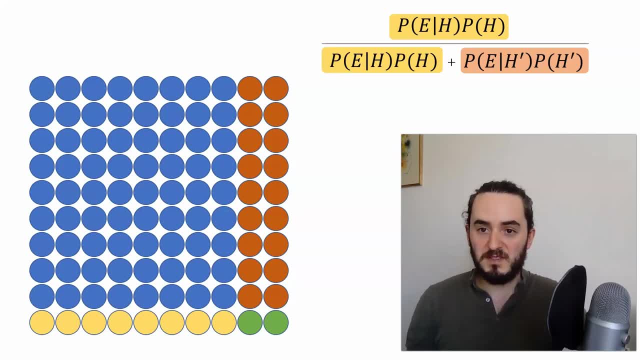 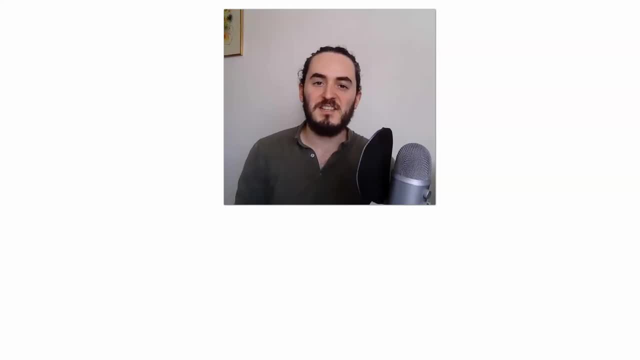 the probability of a positive test result, given that you don't have the disease, multiplied by the probability of not having the disease. Let's now have a look at an example that will help build some detail into our Bayes theorem and even more understanding The example we're going to. 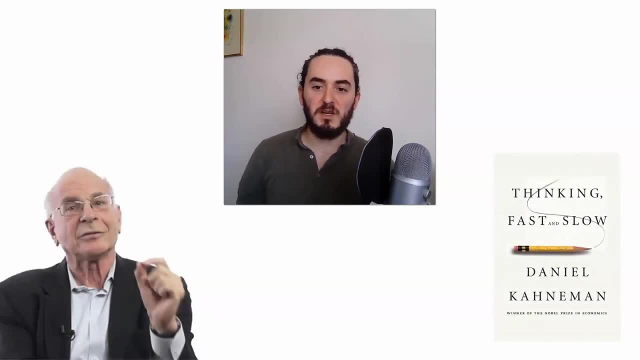 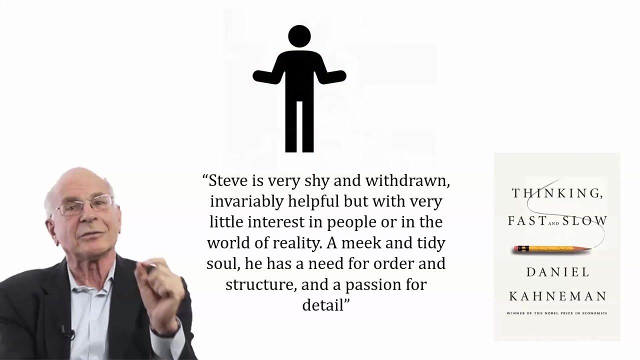 look at is one that was made famous by this guy, Daniel Kahneman, and he talks about it in his book Thinking Fast and Slow, and it's something that he developed many years before with his collaborator, Amos Tversky. So here's the situation we need to consider. Here is Steve, and Steve is very shy and 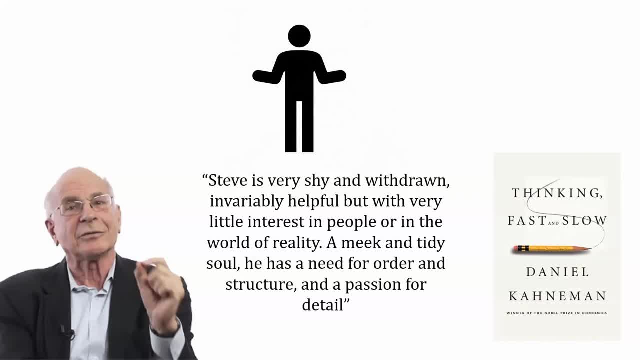 withdrawn, invariably helpful, but with very little interest in people or in the world of reality. A meek and tidy soul, he has a need for order and structure and a passion for detail. Now here's the question that Kahneman poses for us. 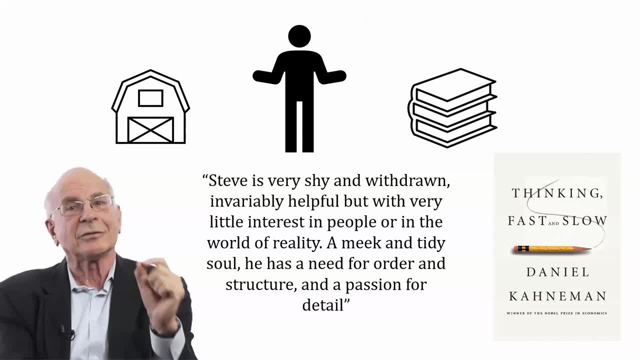 Do you think he's more likely to be a farmer or a librarian? Well, it's obvious, right? He's way more likely to be a librarian. This is everyone's intuition. Let's see if we can use Bayes' theorem to undermine this, to actually figure out what's going on in more detail. So the thing that we 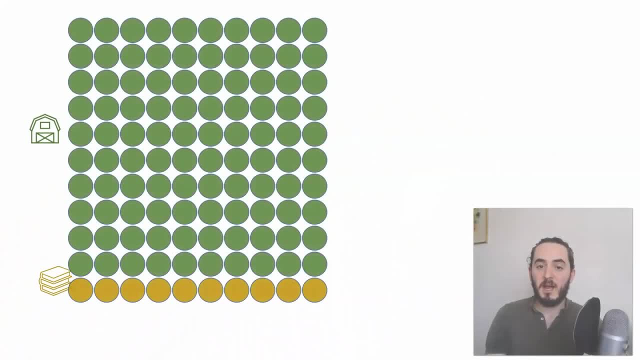 all forget to do is to consider how many farmers and how many librarians there actually are. Now, the precise numbers don't matter, but there are way more farmers in the world than librarians. In fact, in pretty much any country, wherever Steve's from, there are probably more farmers than 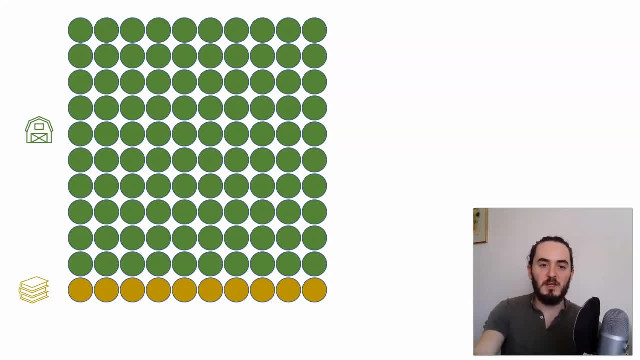 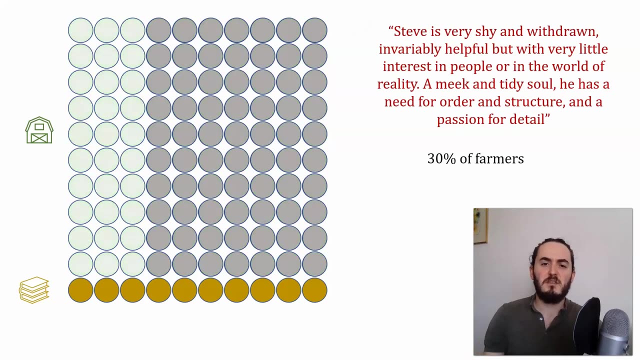 librarians. In my example, there are 10 times more. So here's the evidence about Steve. He's shy and withdrawn and he's helpful and he's tidy and he's meek and he likes order and structure. So we could say: well, what fraction of farmers? Well, let's say it's 30%, Let's say it's a fairly 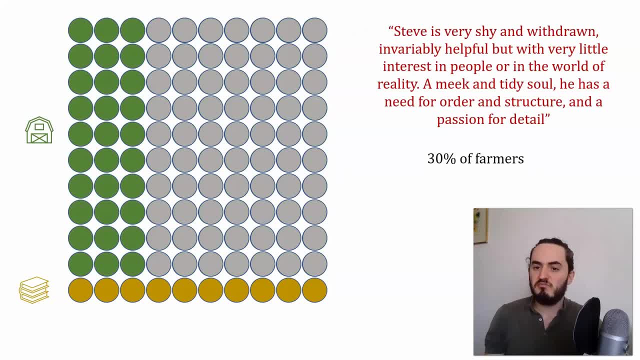 low percentage of farmers. So we could say: well, what fraction of farmers? Well, let's say it's 30%. Let's say it's a fairly low percentage of farmers that meet this criteria. Now it's going to be much more likely among librarians, So let's say that 90% of librarians meet this condition. Well, 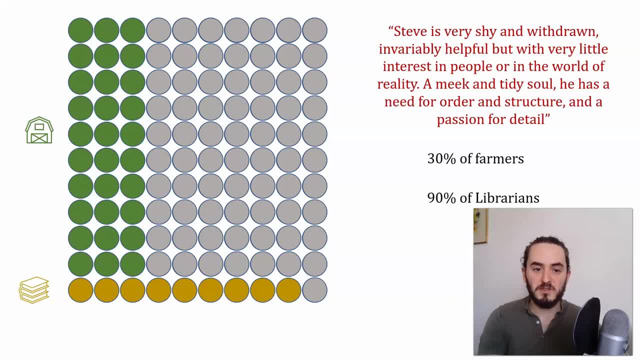 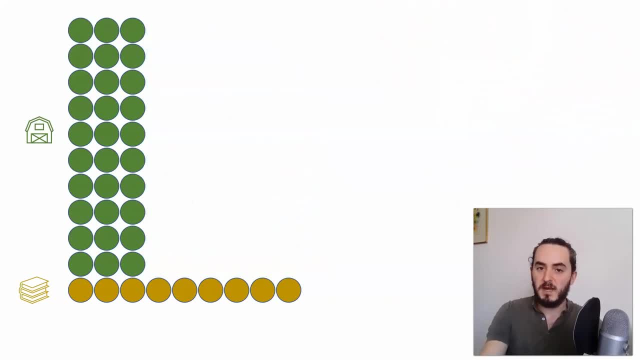 Steve must be either one of the green farmers or one of the yellow librarians. Okay, because they're the people who meet that condition. Well, we now know that Steve must be in one of these groups, So we could maybe look at the ratio. 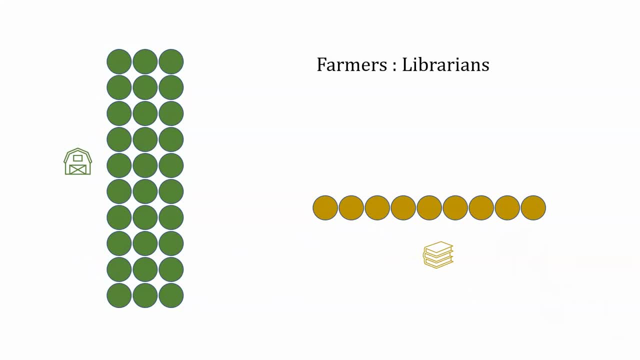 What's the ratio of the farmers, who are meek and tidy and shy, to the librarians, who are meek and tidy and shy? Well, what is it? Well, it's 30 to 9 in my example, to 77% to 23%. So is he more? 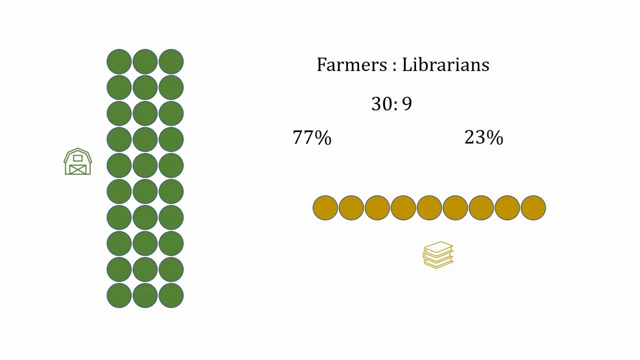 likely to be a farmer or a librarian, Much more likely to be a farmer, And this goes against our intuitions, because the thing that we forget is how many farmers there are. So let's see if we can phrase this all in one sentence. So let's say that 90% of librarians meet this condition. Well, 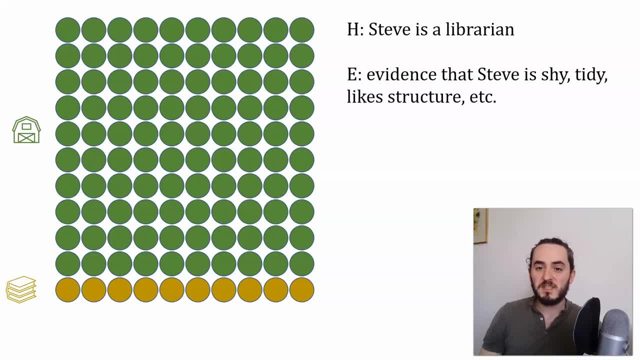 in terms of Bayes' theorem. So our hypothesis, the thing that we are investigating maybe is: is Steve a librarian? And ultimately we want to know, given the information, what's the probability that he's a librarian? Our evidence is that Steve is shy and tidy and like structure. 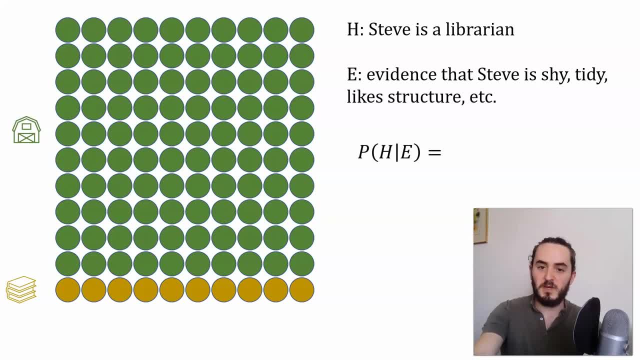 and all of that stuff. So here's the question: What's the probability that he is a librarian, given all of that evidence? How do we calculate it? Well, we first take the probability that he is a librarian. that's our prior probability. that's what we thought the probability is, regardless of any evidence. 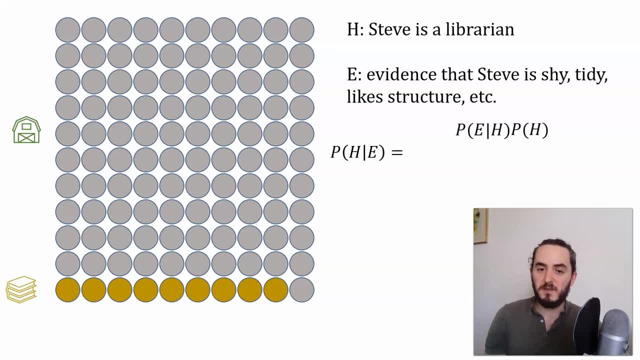 And then we multiplied that by the probability of him being shy and tidy- given that he was a librarians- that shrunk it down from, from 10 people down to nine people, And then we divided that by the total number of people who could be shy and tidy. So that's these same shy and tidy librarians. 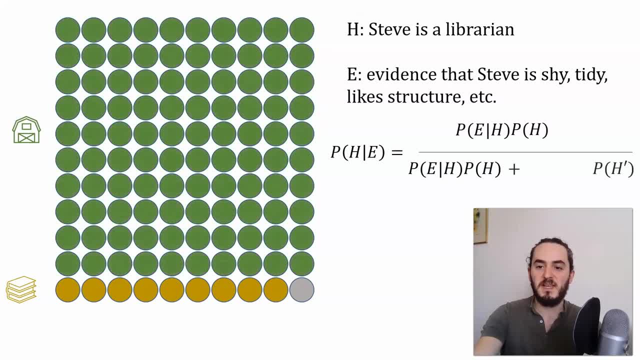 but also the shy and tidy farmers, And we found them by taking the probability that someone was a farmer or not a librarian and multiplying that by the probability of them being shy and tidy, given that they are not a librarian. Okay, let's put some numbers in. So the probability 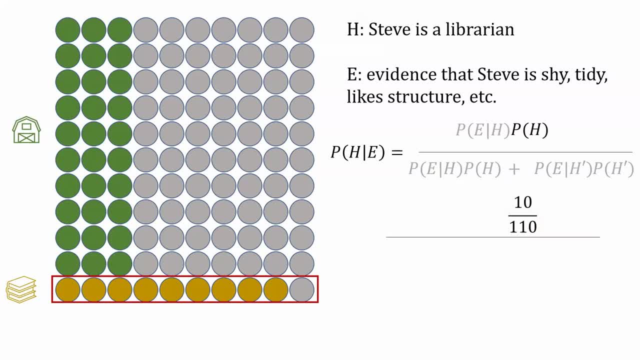 of Steve being a librarian was 10 out of 110.. There are 110 people in the sample and 10 of them are librarians. And then we multiply by the probability of being shy and tidy, given that they're librarians. That shrunk that down by a factor of 90%, So nine over 10 times by. 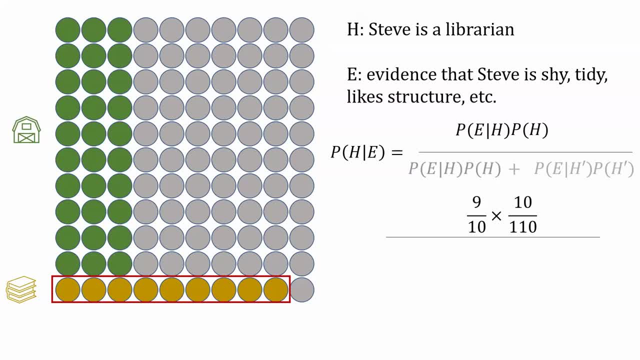 that probability of being a librarian We divided by the same amount again, plus all of the shy and tidy farmers. So we took the probability of a randomly selected person being a farmer- 100 out of 110. And we scaled that down by the probability of those farmers being shy and tidy. So we multiply by: 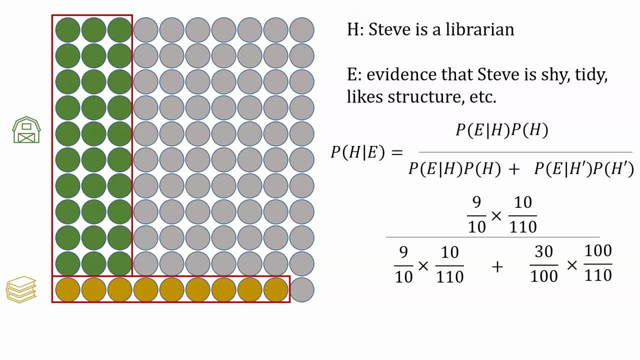 the probability of being shy and tidy, given that you are not a librarian, that is, given that you're a farmer. So those are the numbers. That's how we can apply this to actually plug in some numbers and work some things out, And that's where we get our 23% from. 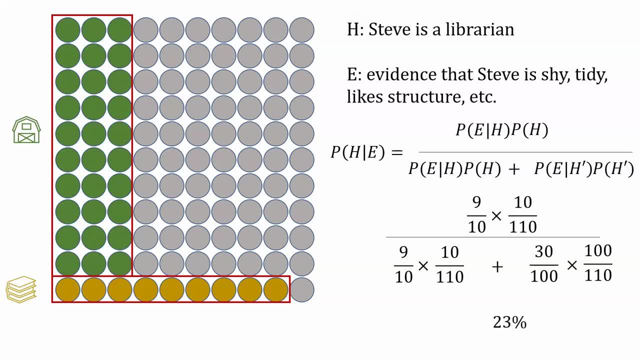 So it's much lower than people think. People hear that information. They think, yeah, I'm pretty sure, I'm pretty sure that Steve's a librarian, but actually he's probably not. He's about three times as likely to be a farmer. Just a word on some of the terminology that's used in relation. 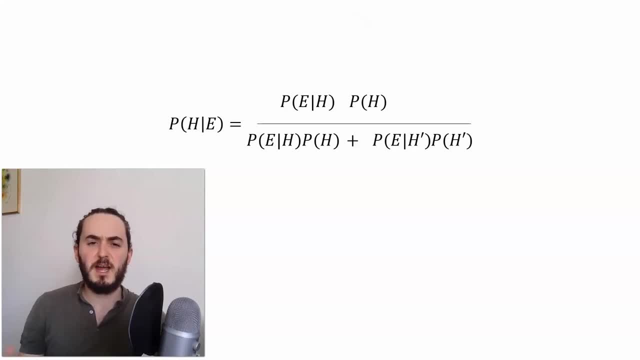 to Bayes' theorem, And I've been using this a little bit as I go, but let's just see how each of these parts is actually named formally. So this bit here- probability that our hypothesis is true- this is called the prior. 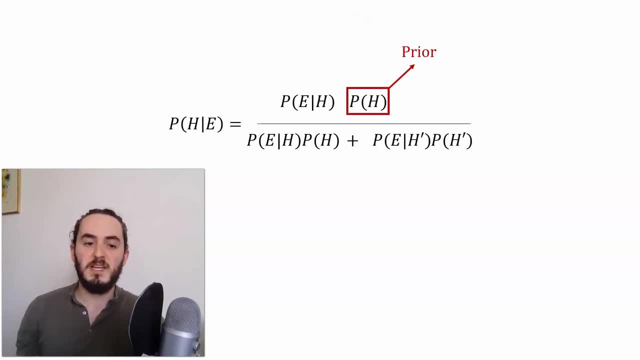 So this is what we think the probability is prior to any new evidence we have. So, in the case of our librarians and farmers, you just think: well, what's the probability? a randomly selected person is a librarian. Well, in our sample it was 10 out of 110.. So that's before we have any. 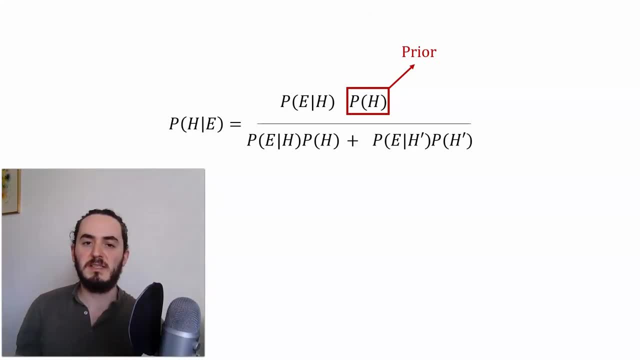 information about the situation. That's what we think the probability is. Now, in contrast to that, this part, the answer is called the posterior, So posterior, meaning afterwards. So, after our evidence, what do we now think the probability is? So there's this contrast of what do we think it. 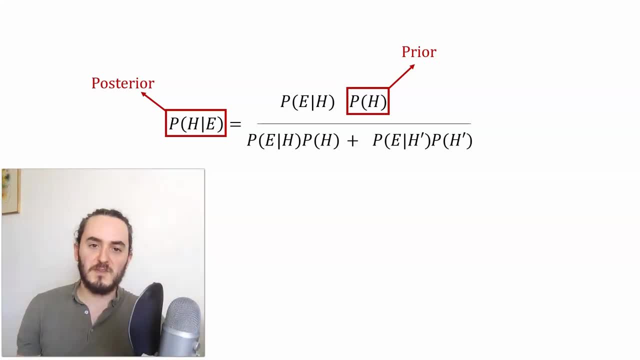 was before we saw the evidence, the prior. What do we think it is after the evidence the posterior, The other parts of this. well, this is called the likelihood, So that's the probability of seeing this evidence, given that the hypothesis was true And in the case of our librarians and 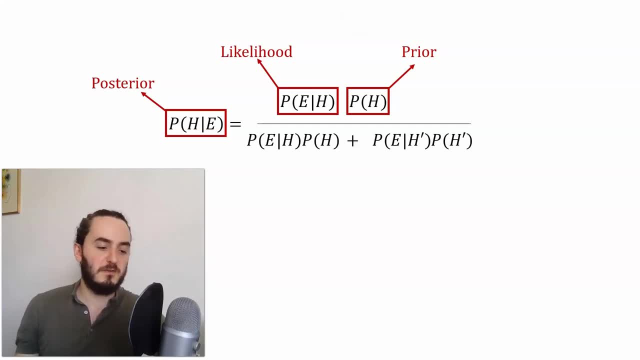 farmers. this is essentially what's the fraction of librarians who are meek and tidy. So this was the 90% in that case. Finally, this whole denominator is called the evidence. It's sometimes called the marginal likelihood. So really, that whole expression. 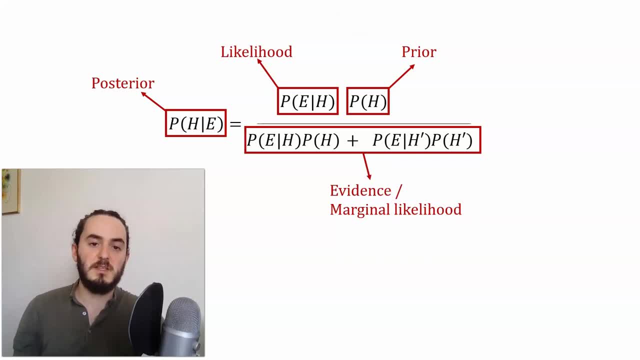 could just be written as probability of E, probability of the evidence. That's what we did in our baby Bayes theorem And it's just the general probability of seeing the evidence that we've seen And it's split up into the chance. 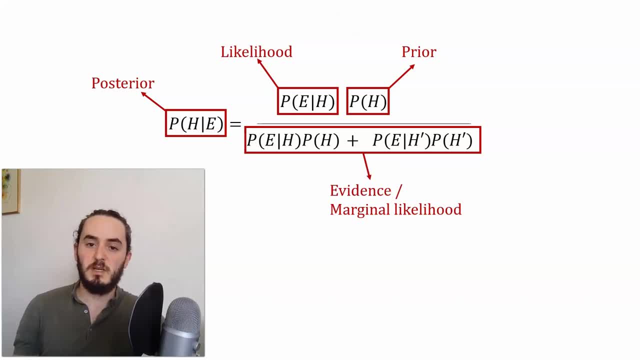 of seeing the evidence if the hypothesis is true, and then also the probability of seeing the evidence if the hypothesis is not true. So that's the kind of terminology that you'll see when you're working with Bayes' theorem, And often it is easier to write it in the shorthand of just 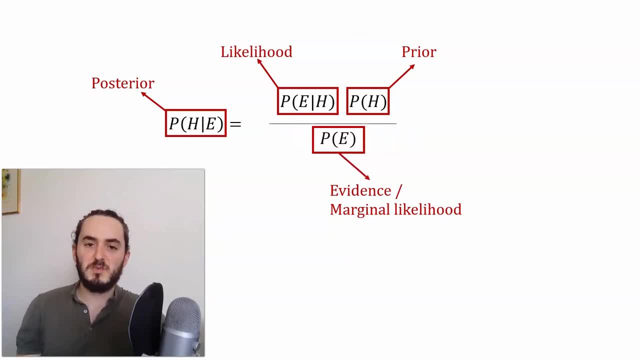 probability of E. but there are situations where the only way you can work out the probability of E is to have it split up into these two groups. So you'll sometimes see Bayes' theorem written like this and you'll sometimes see it written in this shorthand here: 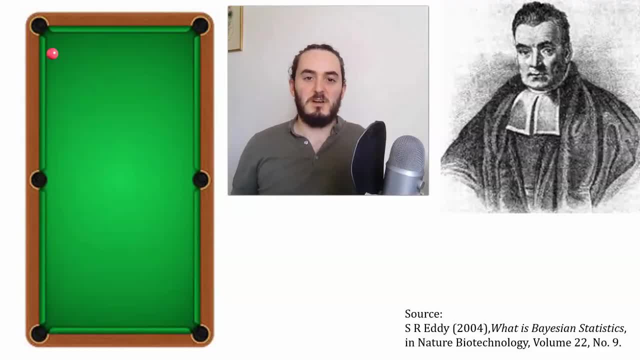 We're now going to look at a substantially more complicated example, but it's a really nice one and it's the example given by Bayes himself in his writings about this when he was first developing this way of thinking. Now I'm adapting this to make it a little bit more simple. 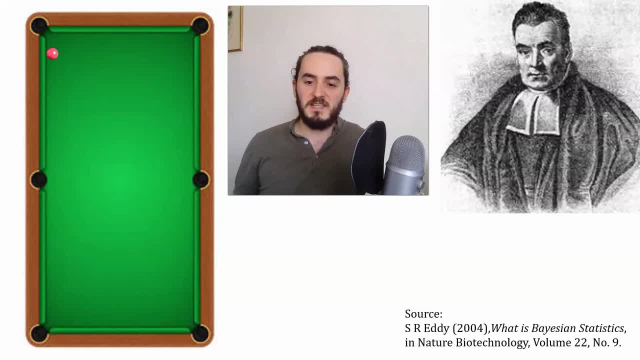 and I'm following an adaptation done by Eddie in his article: What is Bayesian Statistics? So, what is Bayesian Statistics? What we're going to do is we're going to imagine a game between Alice and Bob. Now the game begins by this: A ball is rolled to a random position on the table. What this does? it divides the table. 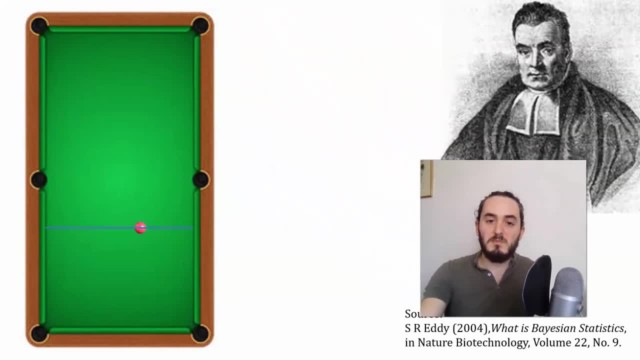 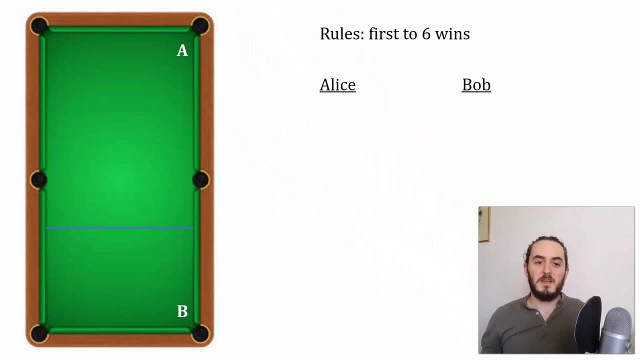 into two sections. Alice and Bob then play the following game. So balls are going to be rolled onto the table randomly. If they land on Alice's side, she gets a point. If they land on Bob's side, he gets a point. 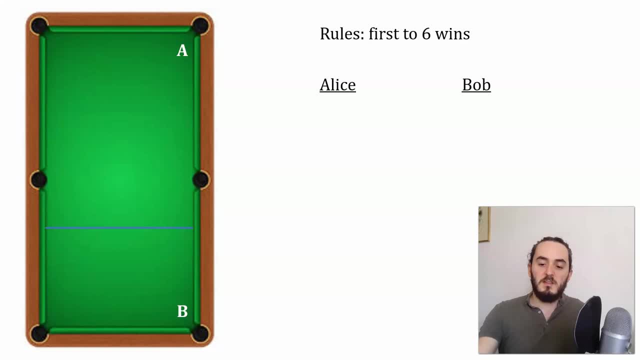 And the rules are: first to six wins. The only thing is Alice and Bob. and let's pretend us. we can't see the table. We don't know how it was divided in the first place. Okay, so we're not sure where that blue line was. So let's say that the game begins and Alice gets. 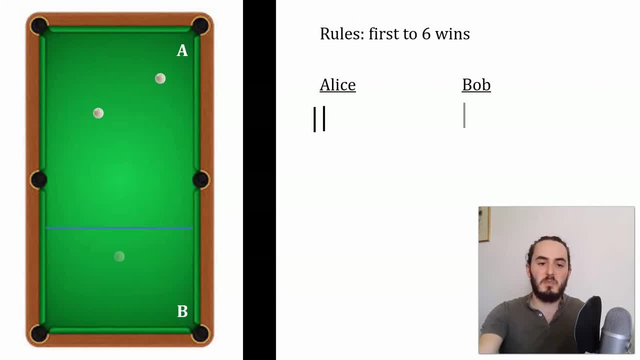 the first point, The ball lands on her side, and then maybe Alice gets another point and the ball lands there. So Bob wins and the game proceeds. Alice gets a point, Bob gets a point. Now all they know is the points they're getting. 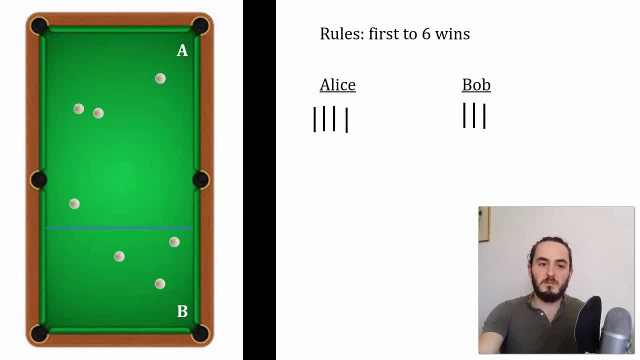 not where the balls are landing. And Bob gets another point, Then Alice gets a point, and then Alice gets a point. So let's pause at this point. What is the probability that Bob will win this game And what should Bob think it is? What should Alice think the probability is, Since they don't? 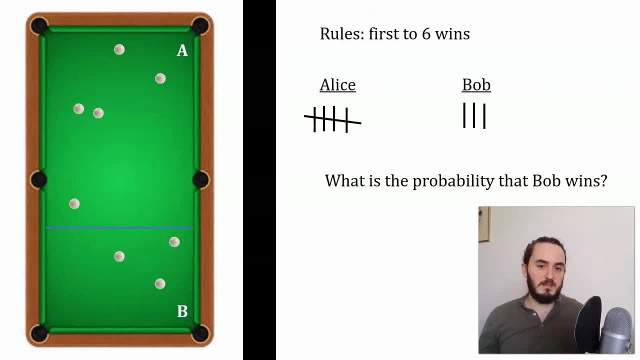 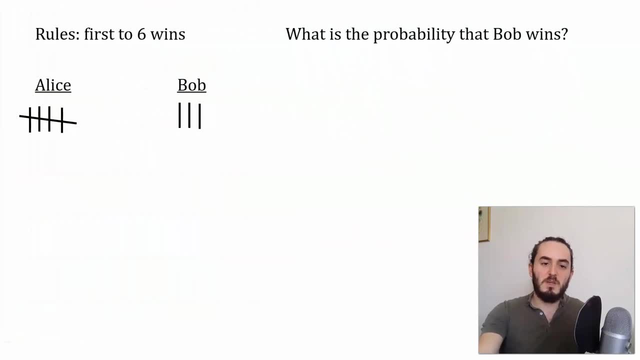 know where the blue line is. they don't know where the other balls landed. All they have are the results. So how on earth can we solve this problem? Well, what's the probability that Bob gets a point on any given go? That's going to be a useful starting point for us to think about. So we'll begin by. 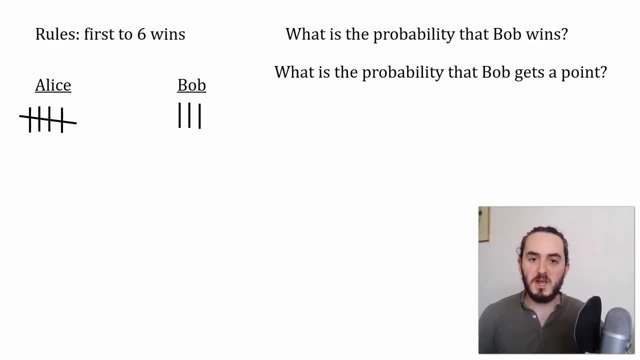 actually thinking about this problem from a frequentist standpoint. If you remember, way back in the first video of this course, we looked at the difference between frequentist methods and Bayesian methods, And this is a great example to contrast them and see how the Bayesian method 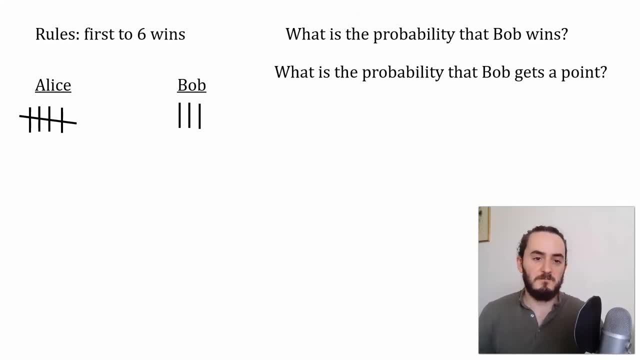 can solve the problem. So here's what the frequentist would do. The frequentist would have no problem answering this question: What's the probability that Bob gets a point? Well, he's got three of the points so far, out of eight goes. So that's what the probability is: that Bob wins a point Now in order to win. 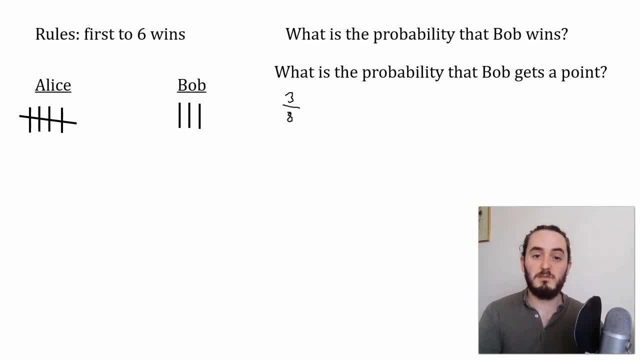 the game he's going to need to win the next three points. So the probability of that happening is three eighths Cubed. So it's pretty simple for the frequentist. They can just carry out that calculation And what we get is about five point three percent. All right, So that's how the frequentist would. 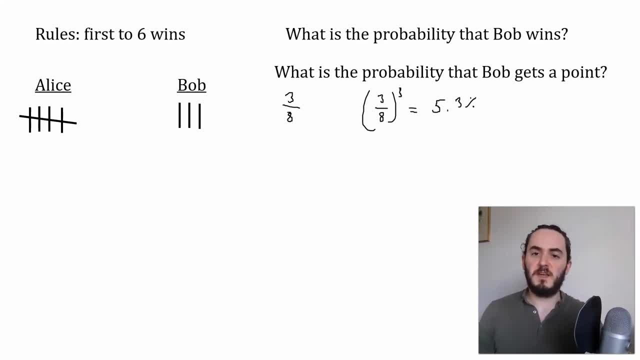 think about it, And there's some pretty good reasons for thinking that this might work. So another way that we could think about it would be this: You could say: well, imagine that the probability that Bob gets a point is three eighths. So that's how the frequentist would think about. 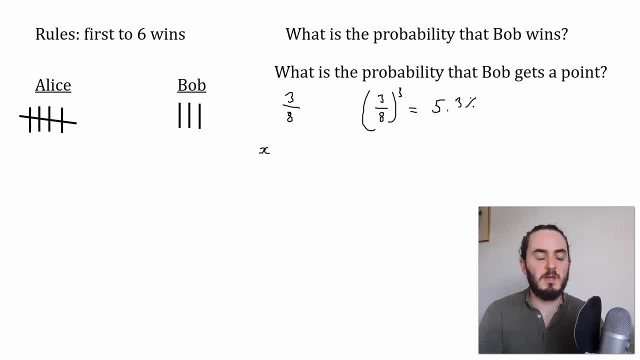 it. So the probability that Bob gets a single point is X. Well then you could say: what's the probability of seeing these kind of results? Well, out of a total of eight turns, what's the probability that Bob would get three of them? Well, anyone who's studied binomial probability 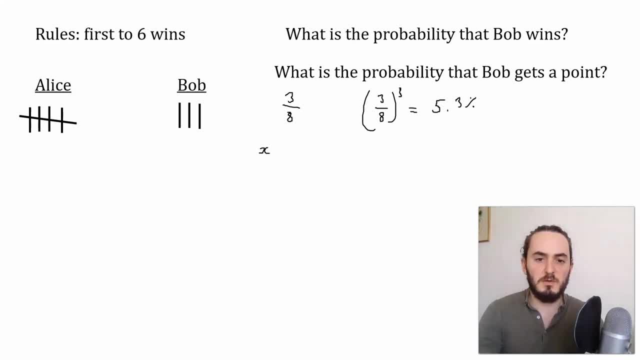 will recognize this as a binomial probability question. So the probability that the number of points that Bob has got is three and the number of points that Bob has got is zero, So the probability that Alice has got is five can be calculated using eight. choose three. Now, don't worry if you've not. 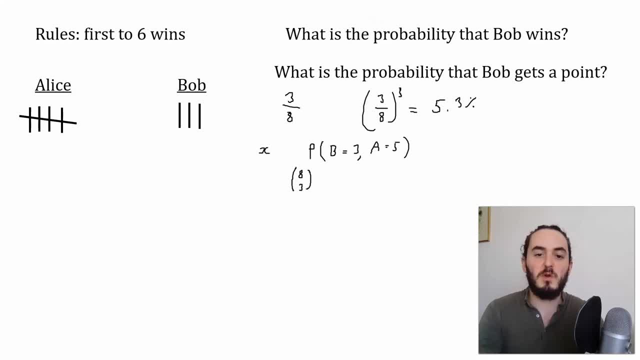 seen this before. This is a binomial distribution for events where there are two possible outcomes with fixed probabilities. So eight choose three ways that it could happen And X is the probability that Bob wins any given point. that happened three times And one minus X must be the probability that 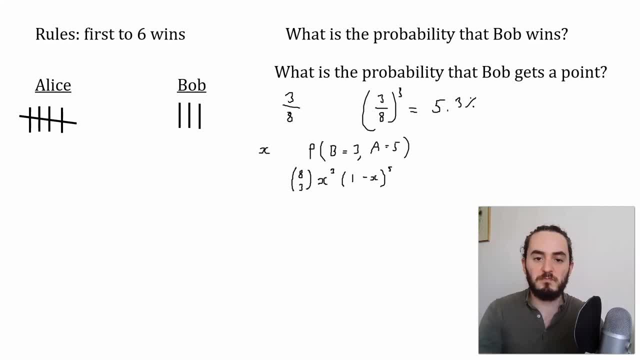 Bob doesn't win or Alice doesn't win, So that's the probability that Bob wins any given point. Alice wins, and that happened five times. So this here is going to give us a function that will give us the probability of finding ourselves at five three to Alice for any given probability And in 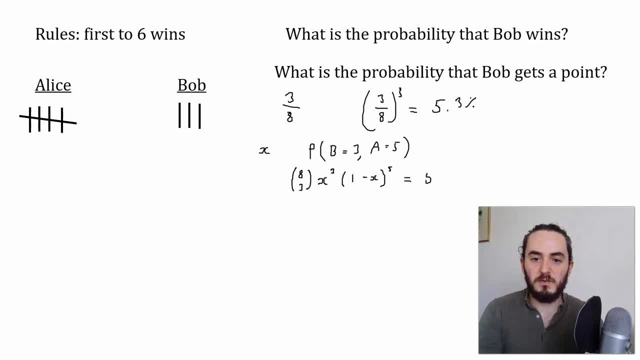 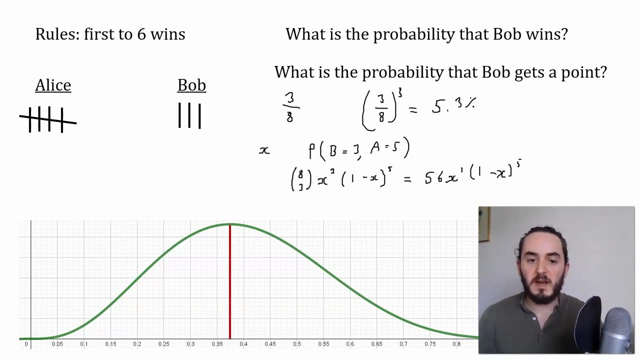 fact, once we calculate the eight, choose three is 56,. we've got this nice looking polynomial. Now we could graph this polynomial, And when we do so, we could say: well, what's the highest point on that? Well, that highest point. 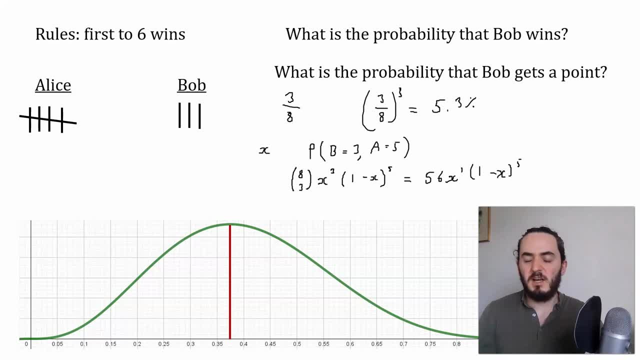 turns out to be three-eighths as well. Now, all of this is just to suggest that the most likely explanation for finding ourselves at a position where Bob has three points and Alice has five points, the most likely explanation for that data, is that the probability of Bob winning each point 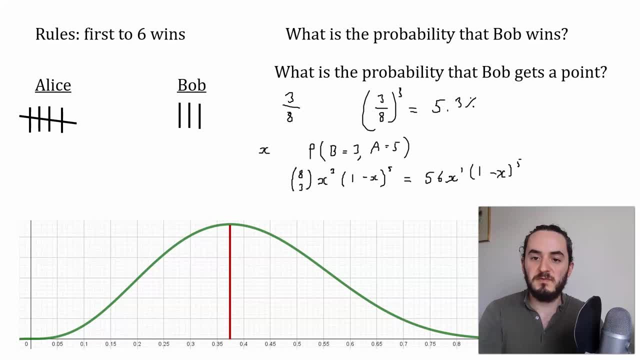 is three-eighths, And if that's the case, the probability that Bob wins any given point is three-eighths. So the probability that Bob wins is five point three percent. It sounds compelling. That's the frequentest approach. Let's have a look at the Bayesian response. So what's the Bayesian going? 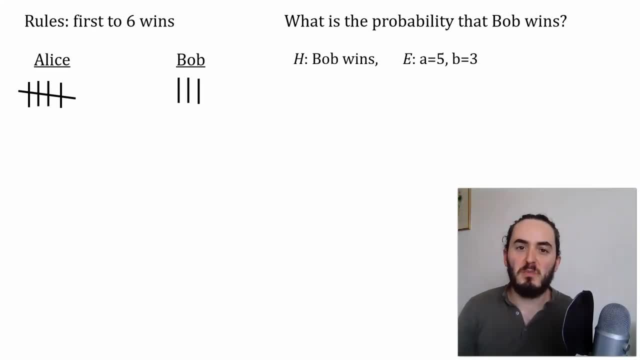 to say with regard to this game. Well, what is the probability that Bob wins? Well, let's use our notation, that's familiar by now. Our hypothesis is that Bob wins the game And our evidence is that the current score is five for Alice And the probability that Bob wins the game is three-eighths. 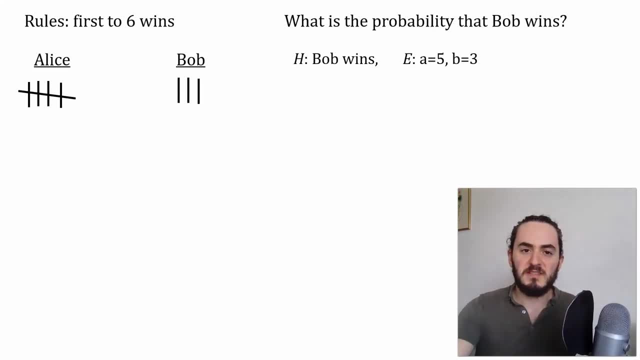 And three for Bob. So let's try to apply Bayes' theorem to this. So what do we know? Well, we know that the probability that Bob wins, given that Alice has five and Bob has three, is- and this is a direct application of Bayes' theorem- it is the probability of seeing a score. 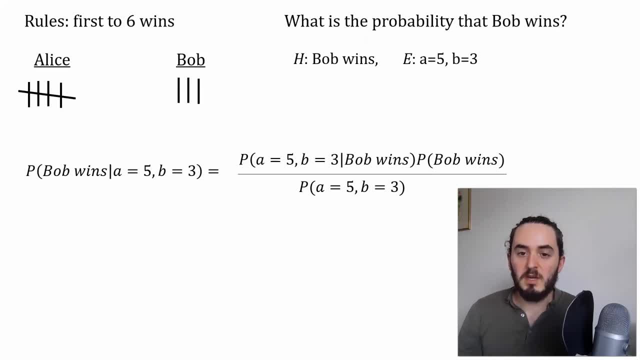 of five-three to Alice, given that Bob wins. multiplied by the probability that Bob wins, divided by our evidence, Which is the probability of finding a score of five, Alice has five, Bob has three. Now I'm going to try to give a sense of how we can use Bayes' theorem for this. I am simplifying things. a. 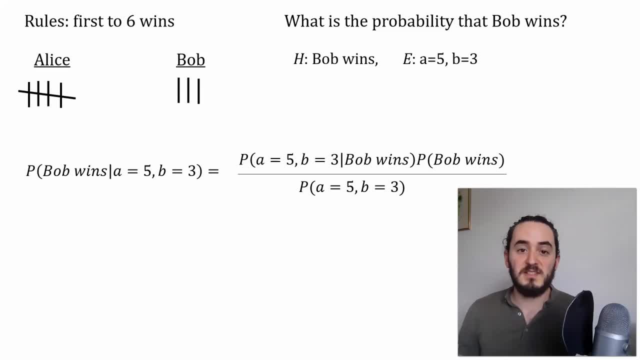 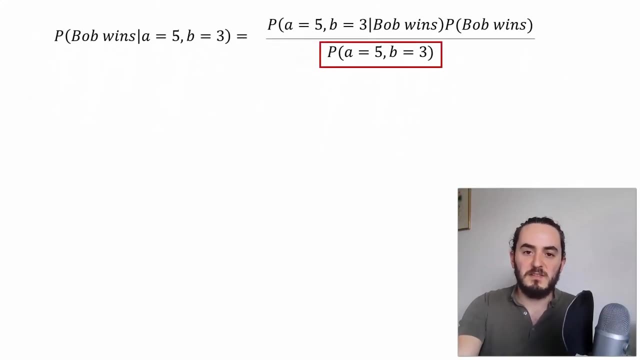 bit, but my aim here is to build some intuitions about how Bayes' theorem can be used in continuous distribution. So we will skip over a few things, but hopefully you'll leave with a sense of how we could extend Bayes' theorem further. All right, let's start then with the denominator. 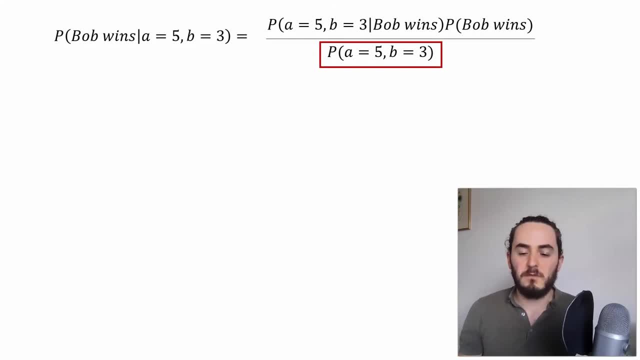 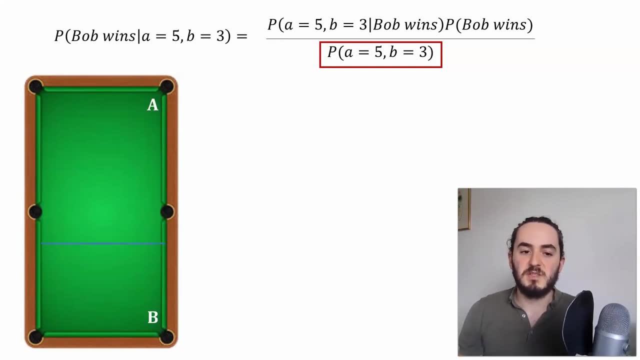 So what's the probability of seeing a score of five-three to Alice? Now, remember that we don't know where this blue line is, So we don't know what the probability is that Bob wins any given game. Okay, it could be really big, it could be really small, it could be anything down to zero. 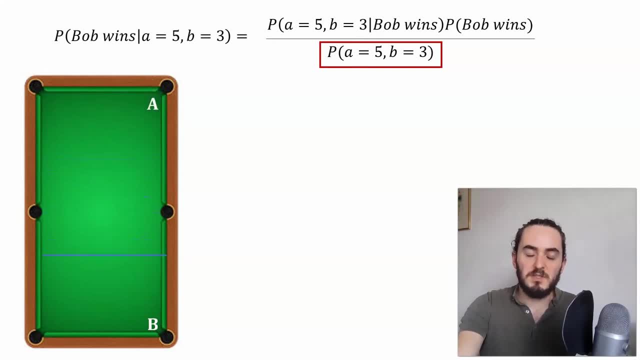 and anything up to one. So in light of that, we're going to have to think: what's the probability of seeing a score of five-three to Alice? So what's the probability of seeing a score of five-three to Alice In general, across any given probability of Bob winning a single point? So let's name that and 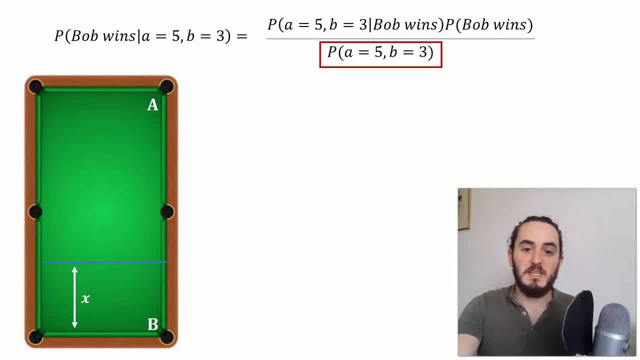 let's call that X. Let's say that X is the probability that Bob wins any given point. We saw from before that the probability of seeing this evidence is a binomial probability. H2 is three times X, cubed times one minus three. So that's the probability And so the probability. 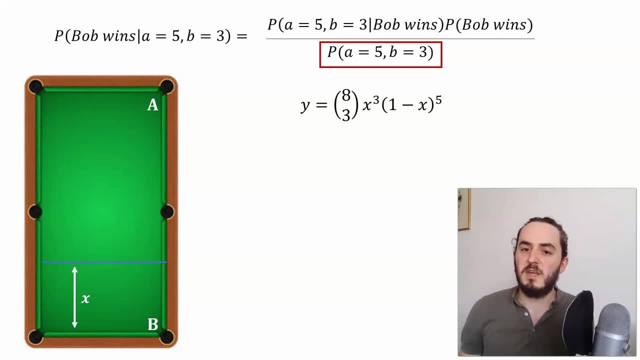 of seeing this evidence is a binomial probability. H2 is three times X, cubed times one minus three x to the 5.. Now we want to know what is the sum of all of these different possibilities for all values of x from 0 to 1.. Now, if you've studied calculus, you'll know that if you have a continuous 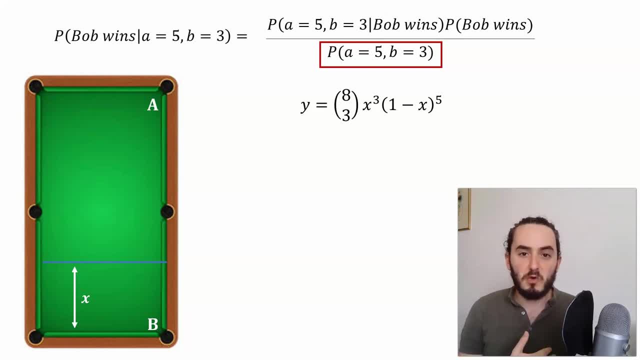 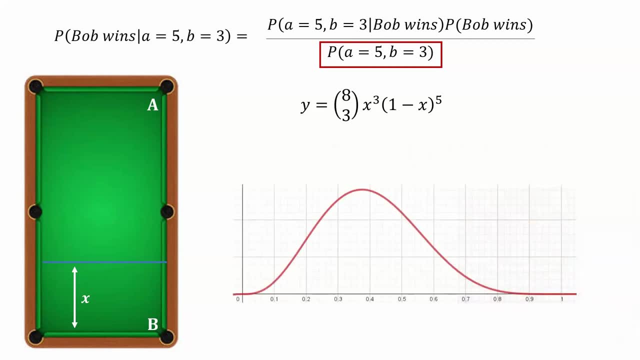 distribution and you want to know what the sum of all possible results is for infinitely many values. we can do that using calculus, So what we're looking for is the integral of this function between 0 and 1. That is, finding the area under the graph will tell us what the probability is. 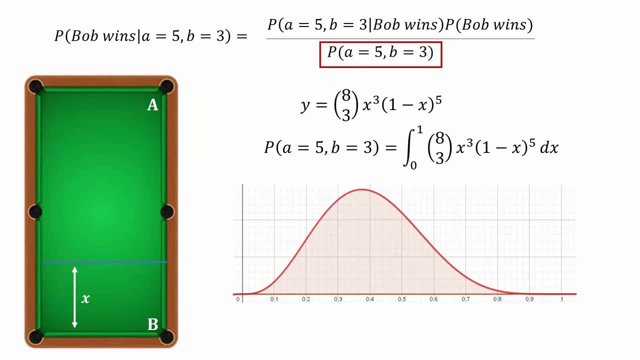 of seeing this evidence of Alice 5, Bob 3 for all possible values of x between 0 and 1.. If you work out that area using calculus or using a computer, you're going to find that it's 1: 9th. So what this tells us is that in general, there is a 1: 9th chance of playing a game of calculus. So what we're going to do is we're going to find that it's 1- 9th chance of playing a game of calculus. So what we're going to do is we're going to find that it's 1- 9th chance. 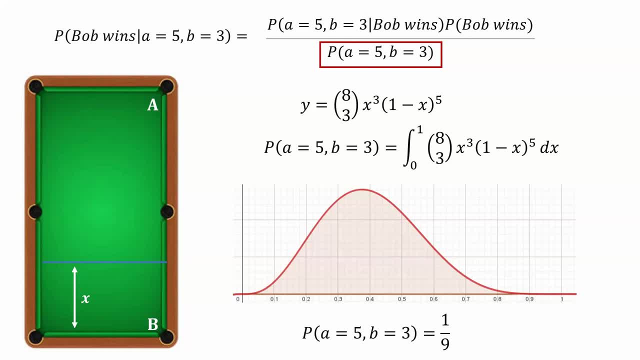 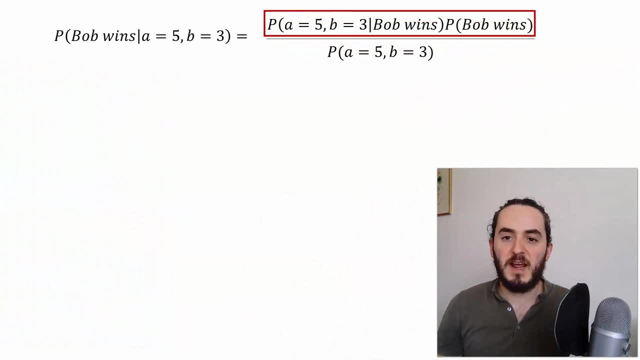 of playing this game and, at some stage in the game, finding yourselves in a position of Alice 5, Bob 3.. Okay, let's move on now and have a look at this numerator. Okay, so this is the part where I will simplify some things, and that's just to in order to aid intuitions. So, this first part, probability. 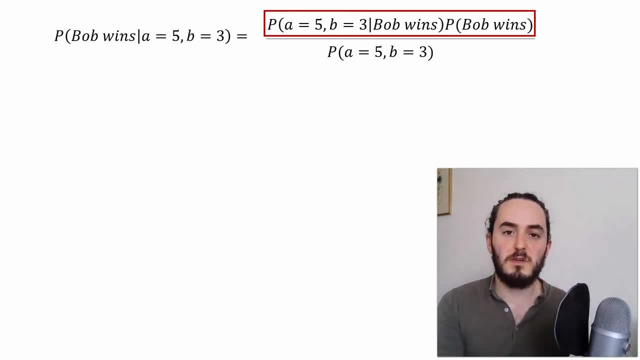 that a equals 5 and b equals 3, given that Bob wins. Well, can we come up with a function that could capture that? Well, we know what the function is. We know that the function that describes Alice having 5 and Bob having 3 is this binomial expression: here 8. choose 3 and then Alice. 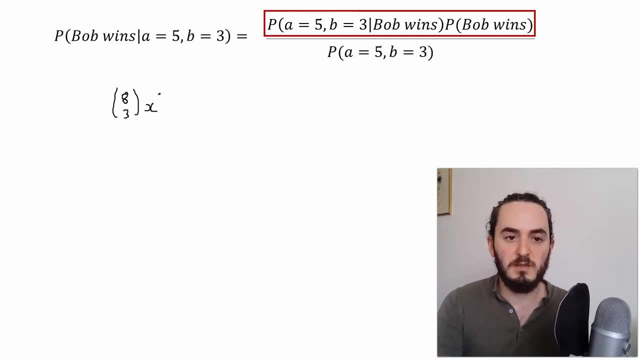 has 5 points. Well, let's do Bob's first. Bob has 3, so x happened 3 times. Alice has 5, so that's 1 minus x and that happened 5 times And that's sort of independent of the fact that Bob wins. 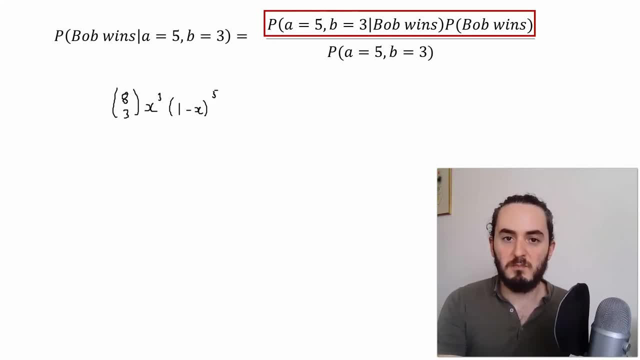 For any given probability for Bob. we know that this expression captures that And I am simplifying, but hopefully this makes some sense. Now, the probability that Bob wins. Well, if Bob is going to go on and win from here, he will need to win the next three games, because it's first to six. 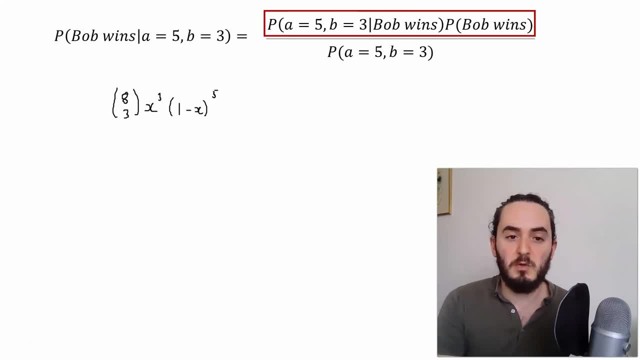 and he has three points. He's going to have to win all of them, which means we're going to need a further x cubed. So that represents Bob winning and Bob winning and Bob winning. Now this expression here, since we've got x cubed and x cubed, can simplify to 8: choose 3, x to the. 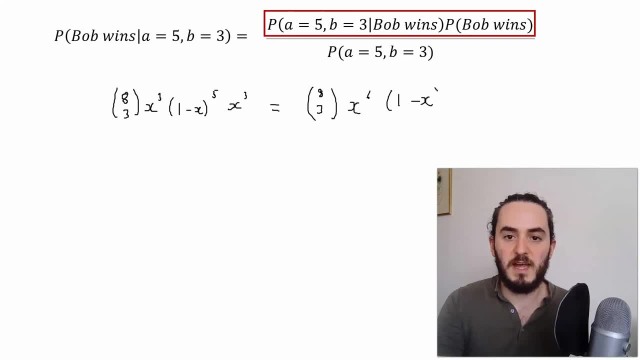 power of 6 and 1 minus x to the power of 5.. So, just as before, in order to figure out what this probability is for all values of x, we'll use calculus. So here is our function that represents the distribution of that numerator, That's of the score being 5. 3 to Alice, given that Bob wins. 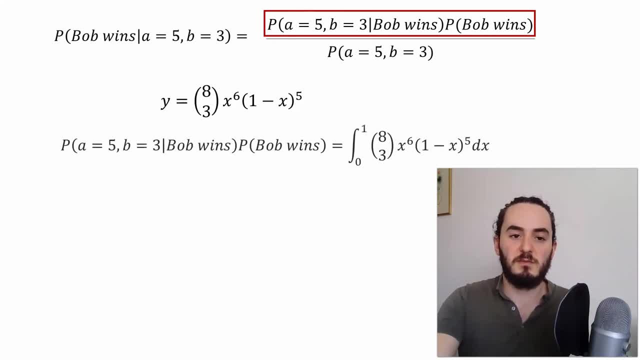 multiplied by Bob, going on to win the next three points. So, in order to do that, it's the integral of this function between 0 and 1 and that's going to capture the area under the curve, The area under that function between 0 and 1.. If you calculate this integral again, you can do that using: 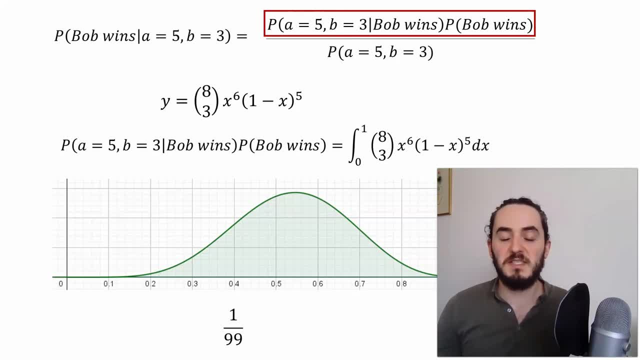 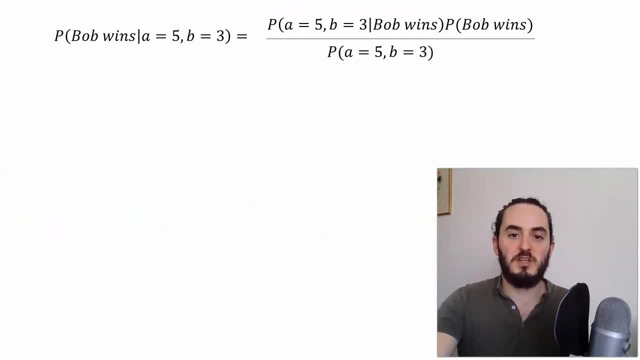 using calculus or using a computer, You get 1 over 99. So now we know the numerator and we know the denominator. It's just a question of plugging those values in. So our numerator was 1 over 99. Our denominator was 1 over 9.. That 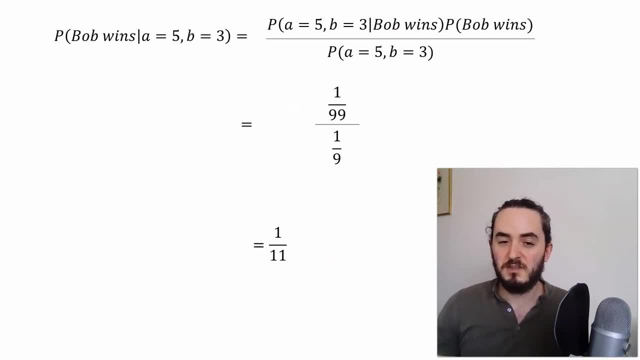 simplifies to 1- 11th. So that's what the Bayesian says. the probability is that Bob wins. So, to contrast the frequentist who just looked at what happened and said: okay, so Bob's chance of winning each point is 3- 8ths. 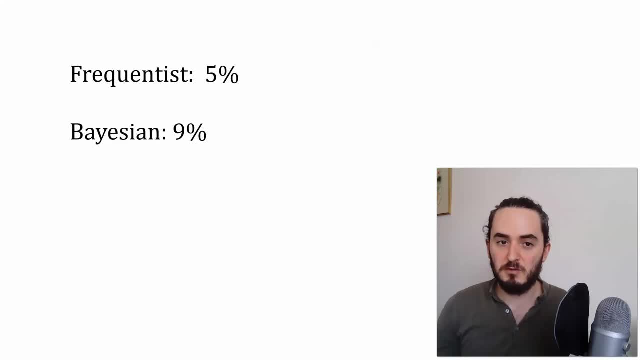 The probability is 3, 8ths cubed. It's easy to do, but it gives us an answer of about 5%. Using this much more complicated Bayesian approach gives us 9%. It's almost twice as much. Now, I think everyone's response to this is to say: okay, but who's right? Well, in the next video I'm going to 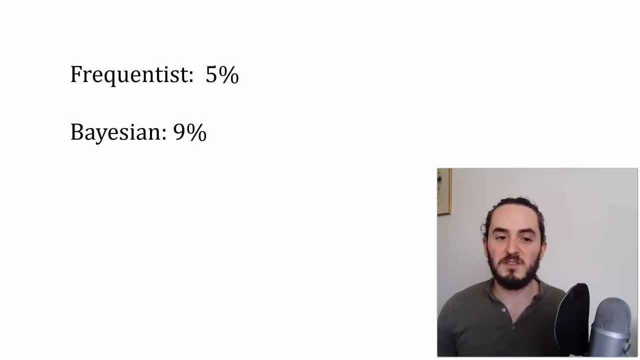 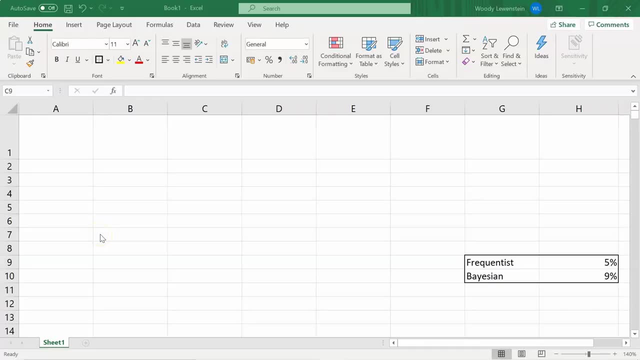 go through a simulation that hopefully can give some evidence that it's true. So I'm going to go through a simulation that hopefully can give some evidence that the Bayesian has got this one correct. All right, so in this video we're going to use good old Excel to test who was right. So remember what? 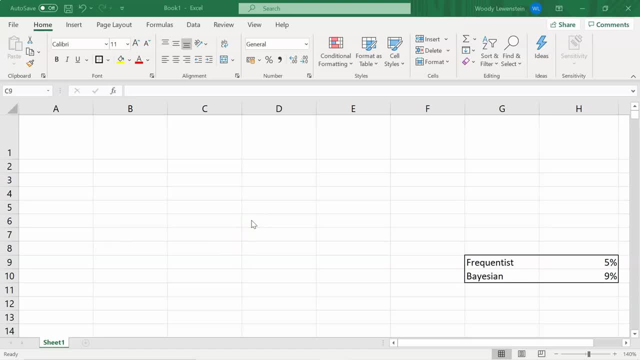 the situation was Given that we found ourselves at a position in the game where Alice was 5-3 up. what's the probability that Bob goes on to win? The frequentist said the answer was 5%. The Bayesian said the answer was 9%. I'm going to set up a simulation here where we're going to 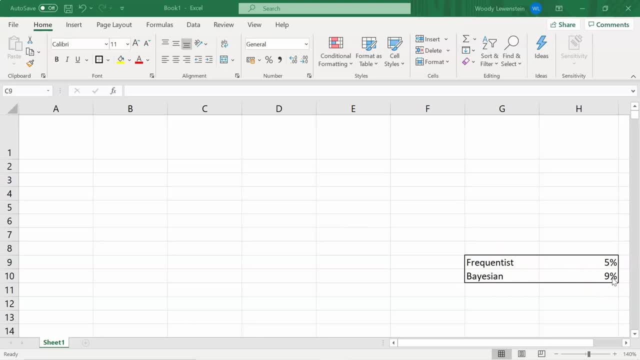 simulate thousands of games many times and see what actually happens. Okay, whose answer was closest to what happens in our simulations? That should give us some sense of who's correct. So the first thing I want to do is just to say: well, what was Bob's chance of winning on any given? 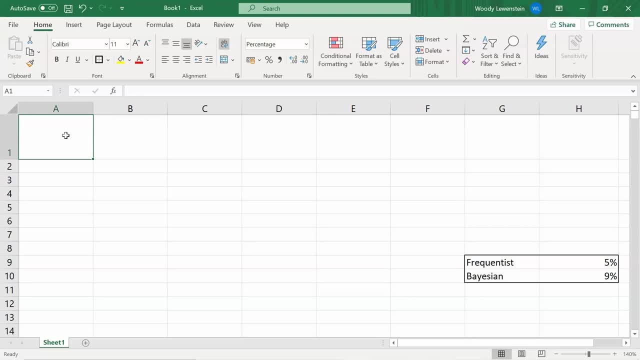 game on any given term. So really, where did that initial ball land? So that's Bob's chance, Bob's chance of winning any given point. and this is just a random number between 0 and 1, and I'm expressing that as a percentage here. So let's just generate. 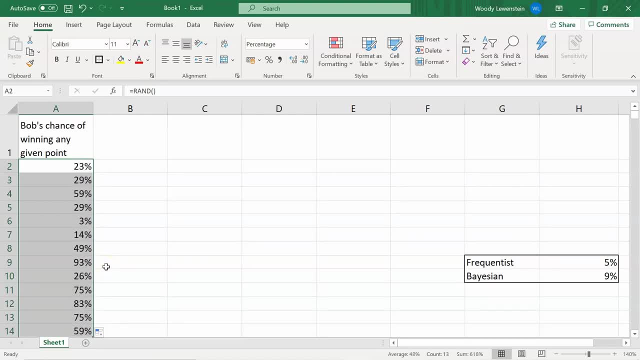 a few. So there we go, and each time I click a button I can just regenerate. So those are some different probabilities for Bob winning a point. Now the next thing I want to know is what's the probability of reaching Alice 5, Bob 3? Did the game actually reach 5-3 to Alice? So the first. 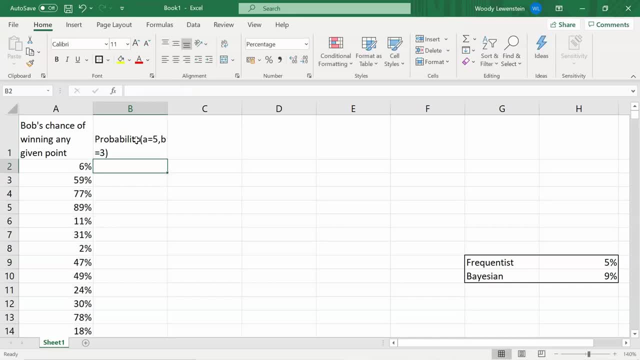 thing I want to know is what's the probability of reaching Alice 5, Bob 3?? Well, that's a binomial probability which we discussed in a previous video. So what's the probability? Well, the number of times that Bob should have won is 3.. There were 8 games if we got to 5-3, so out of 8 trials, The 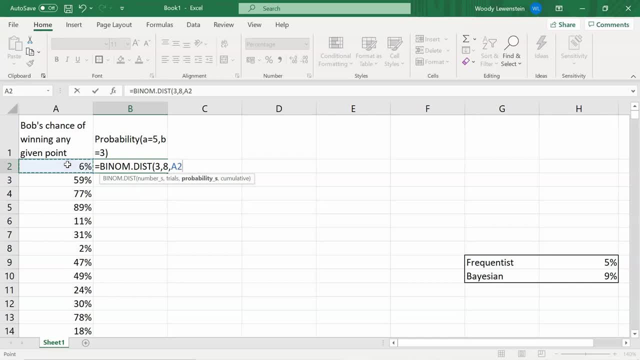 probability of Bob winning any of those was the number we generated here and it wasn't cumulative. it's not the probability of winning anything up to 3, it's winning exactly 3.. So now we've got probabilities of the game reaching 5-3.. So you can see that when Bob was 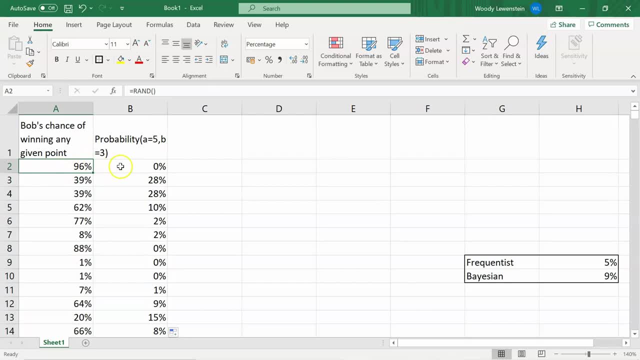 highly likely to win every point, it's very unlikely that we should find ourselves 5-3 to Alice. But in a situation where Bob is about 39% likely to win any given point, it's more likely that we reach 5-3 to Alice. Now, did it actually happen? Did we actually? 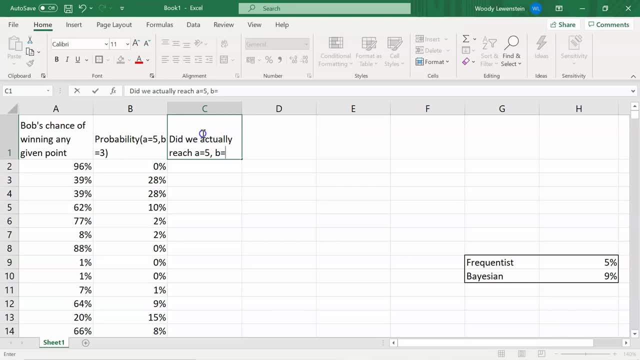 reach Alice 5, Bob 3?. Well, these are the probabilities of it happening, and a really nice way to just randomly see if it did happen is to say: if some new random number is less than what we got here, then yes, it did. 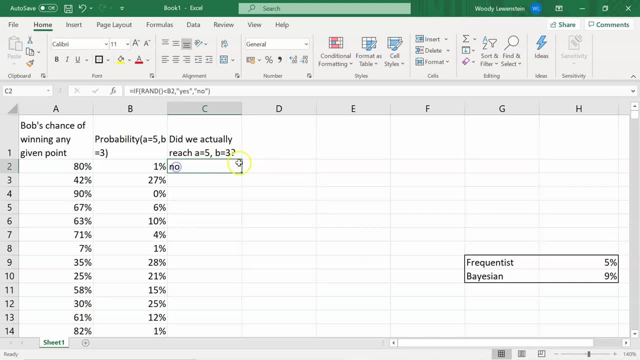 Otherwise. no, it didn't. So now I can see of these games. okay, here's a time where it did happen. So Bob had a 40% chance of winning each point. so the probability of the game reaching 5-3 was 28% and it did. 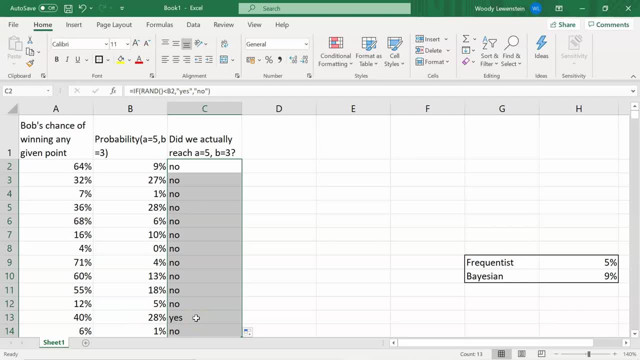 actually happen this time. Okay, so ultimately, we're only going to be interested in the games that did reach 5-3 to Alice, like this one here. So we kind of want to ignore all of the others, which we can do. So what we want to know now is, if it did reach that point, what's the probability that Bob goes? 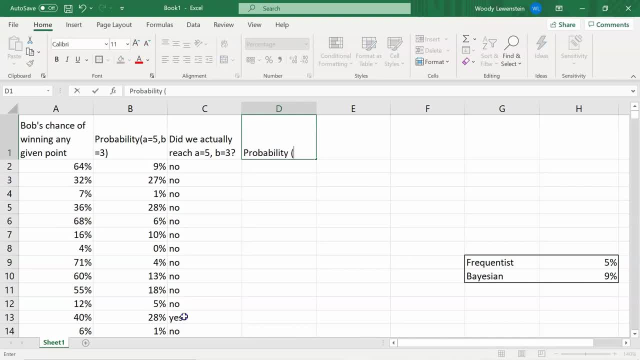 on to win. So this is the probability that Bob goes on to win. So the first thing to do is to say: if this is no, so if it didn't actually reach 5-3 to Alice, then just do nothing, leave the cell blank. 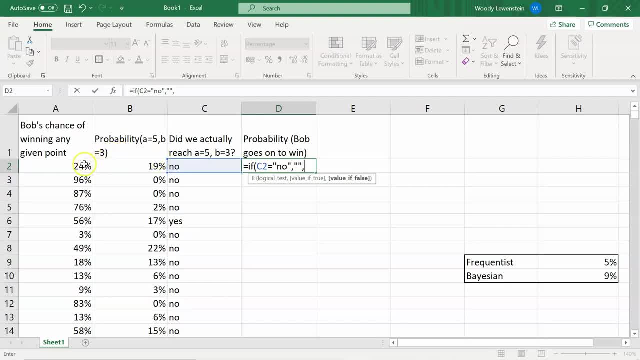 Otherwise, what's the probability of Bob winning? Just whatever his probability of winning? each point was cubed because it needs to happen three remaining times. Well, this is blank because we never reached 5-3 there and none of them did there. but here we go. 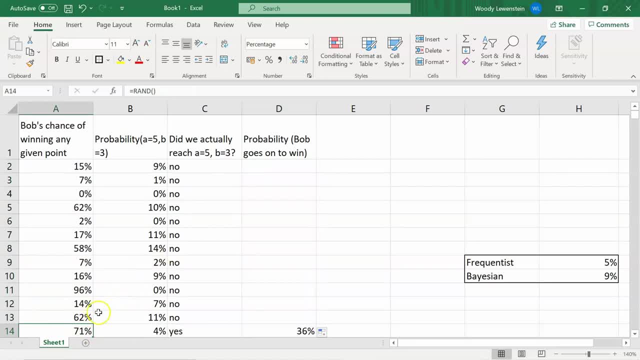 So in this simulation Bob had a 71% chance of winning each point. so the probability of it reaching 5-3 to Alice was only 4%. but it actually did happen in this simulation. but then Bob did go on to win in that simulation. 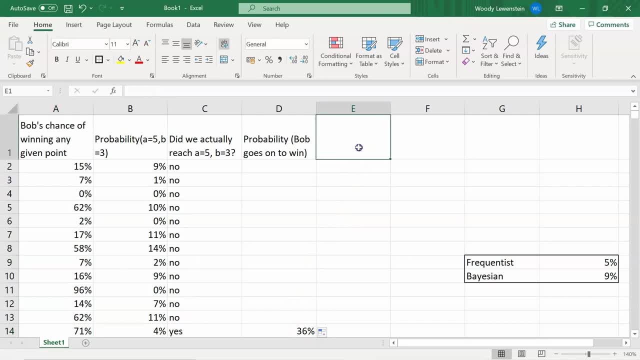 All right, and now we want to know: did it actually happen? So did Bob actually go on and win? Well, we do want to say that if this was blank, then we'll make this one blank as well, because we're not interested in the games that didn't reach 5-3, but otherwise we can do a little. 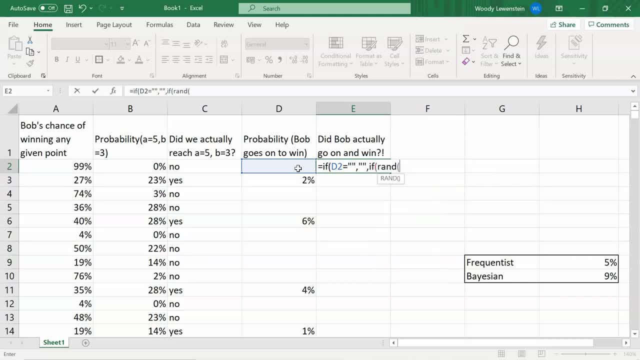 random number check to say If we get into 5-3.. if a randomly generated number is less than the number we see here, then Bob did go on to win, otherwise Alice went on to win. okay, so in this first game let's just generate all of these. 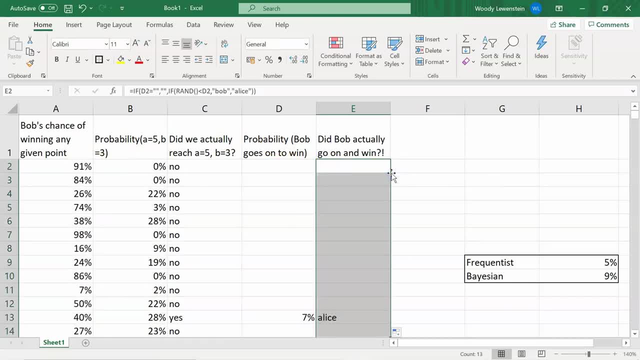 let's wait until there are a few, okay, so in, let's have one. where there's, there's both. there we go. so, um, in all of these blank ones, these were games that never actually reached 5-3 to Alice, but in this game Bob had a 70% chance. 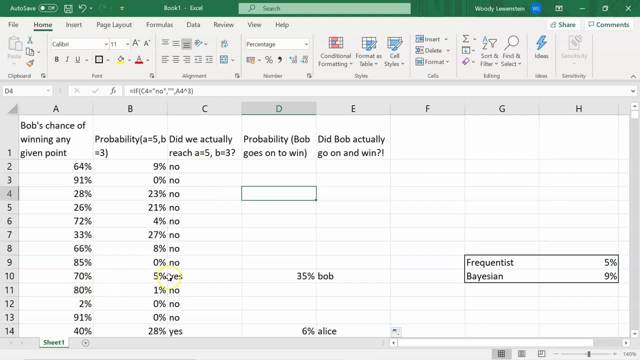 of winning each point. the game did reach 5-3 to Alice, so Bob had a 35% chance of going on to win, and he did in this one. Bob had a 40% chance of winning each point, um the game did go on to reach. 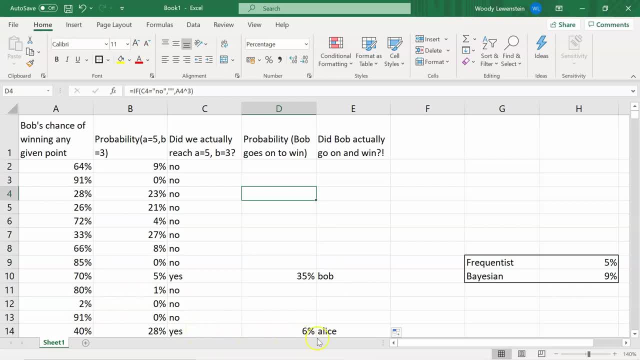 5-3 to Alice, but in that one Bob failed to go on to win and Alice won. so now our question is: what's the trend then if we were to do this loads and loads of times? how many of these games that reach 5-3 end up with Bob winning and how many with Alice winning? 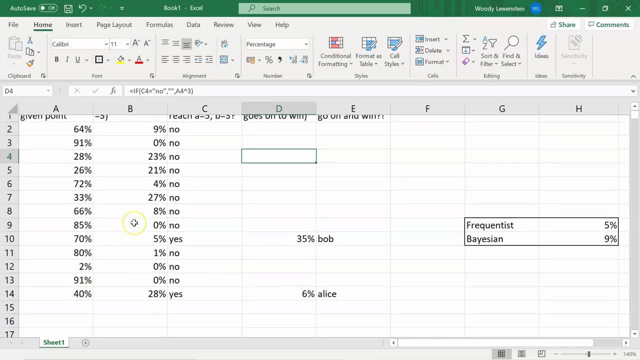 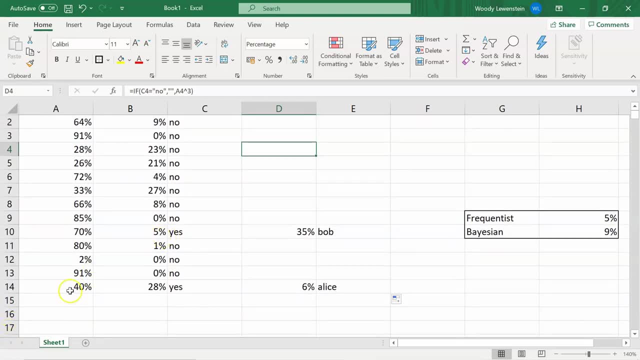 well, to do that, we need to generate more than how many we've got now. we've got 13, so let's do that. let's generate way more now. how many of these games that reach 5-3 end up with Bob winning and how many with Alice winning? 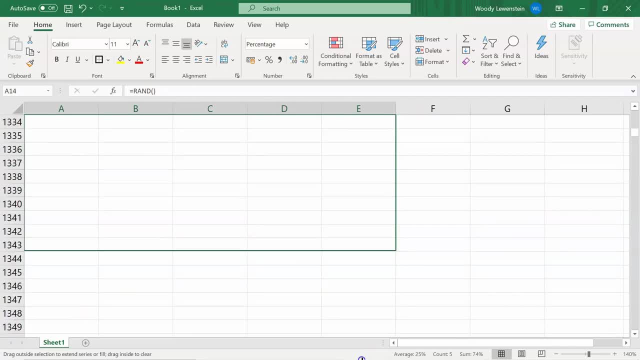 how many is enough? that's a pretty good question. um, generally 10,000, I mean, depending on what you're modeling. 10,000 simulations is a is a decent start. anything less than 10,000, you're probably not going to get that reliable results. so let's just generate absolutely loads of these. 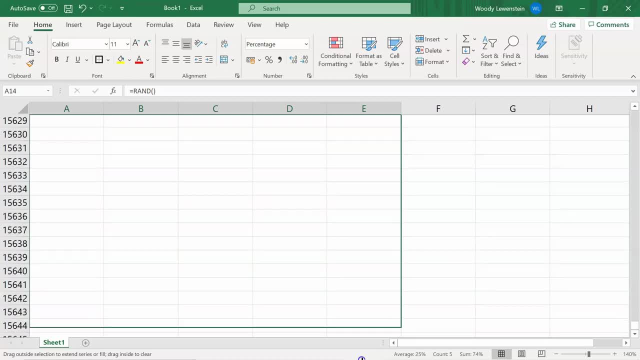 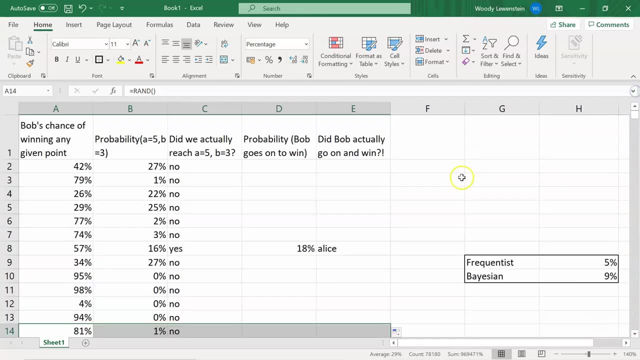 games. so poor old Alice and Bob are spending, you know, years and years playing this game. all right, so that should do so. that's what around 15,000 um games that we've got. so let's do that, let's do that, but obviously the vast majority of them never actually reach 5-3, so we have no result. 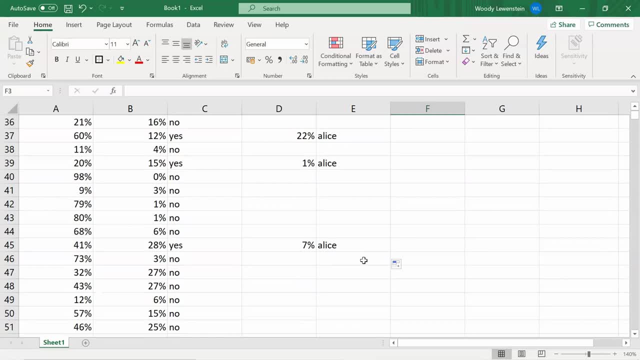 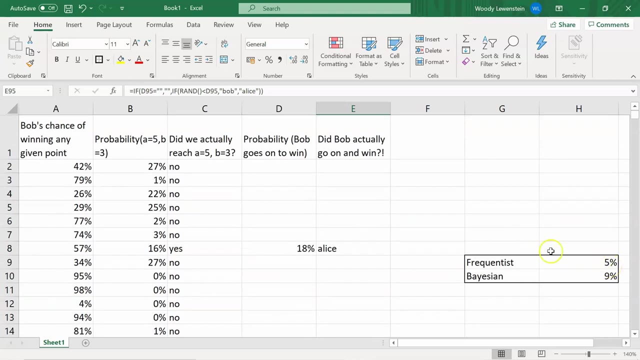 what we're interested in is in this column. it's clearly more common for Alice to win, but what's the probably, what's the proportion of these games that Bob went on to win? is it five percent, as the frequentist says it is, or is it nine percent, as the Bayesian says? 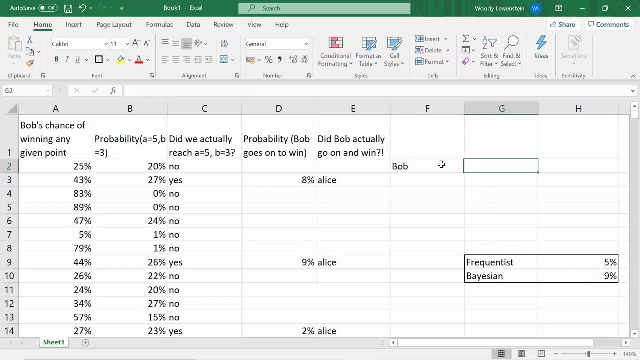 well, we can count this way. so the number of games that Bob goes on to win, I can say count, if in this column you see the word Bob. okay, so Bob, uh, out of all of the games done, Bob won 157 of them and that number is going. 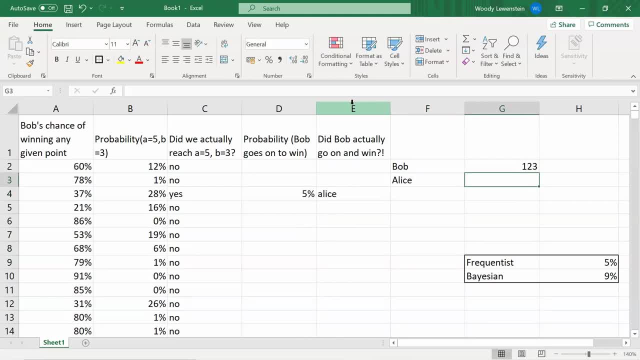 to change every time I do run another simulation. what about Alice? well, I can say count if you see the name Alice in this column. okay, so Alice has won way more, but what's the probability of Bob winning? so the probability of Bob winning, given that the game did reach Alice: 5 Bob. 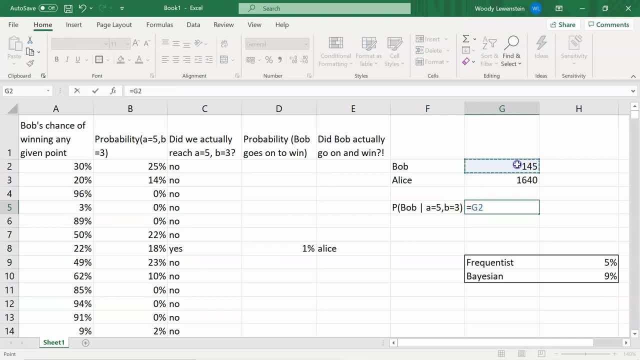 3 is the number of games that Bob won divided by the number of games, which is the number that Bob won plus the number that Alice won. all right, so what do we get? eight. let's convert the two percentage, make it easier, in fact. let's give it a little bit more accuracy. there we go, so. 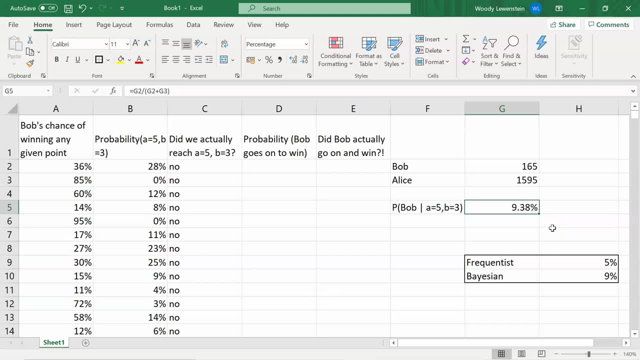 0.2 percent at a time. let's simulate again: nine a bit percent, 8.6, 9.2, 7.8. okay, so it does vary, as we'd expect, with the simulation, but does it seem to be varying around the frequentist answer of? 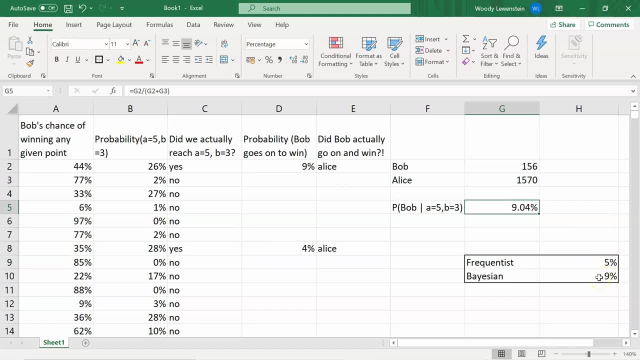 five percent, or does it seem to be varying around the Bayesian answer of nine percent? it's pretty obvious that this is varying around the Bayesian answer of nine percent, and what this suggests is that if I was to simulate maybe a million times, we would very reliably get nine percent. 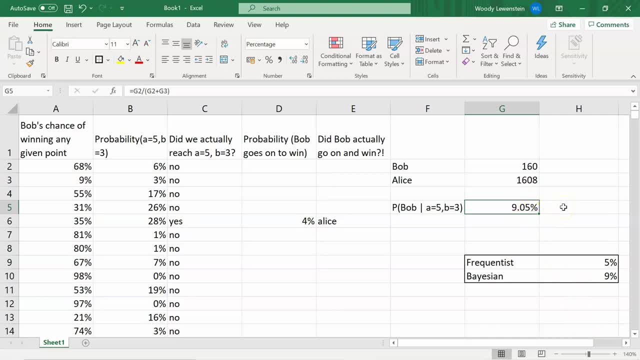 as an answer. that's called the law of large numbers, that the greater the number of simulations, the more this will tend towards the correct answer. so running a simulation like this can give us some pretty compelling evidence that the Bayesians are the ones who've got this right. the 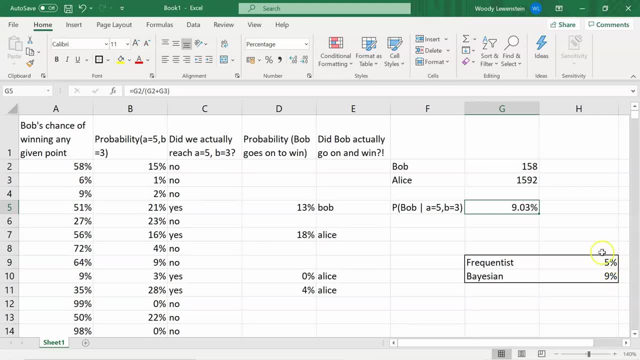 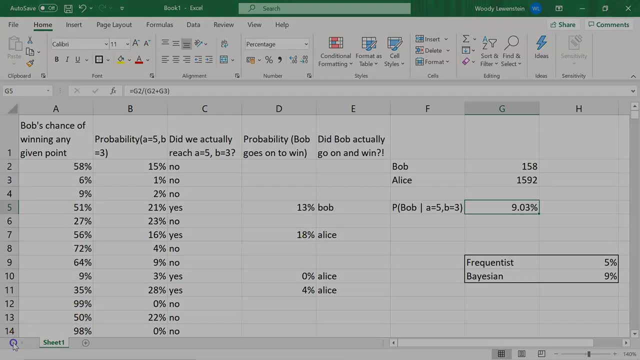 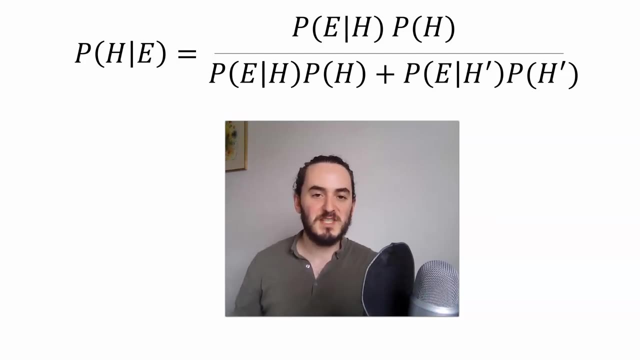 Bayesians who said it was nine percent are not the frequentist. so there we go in as I said they would at the start of the course. there we go. I really hope you've enjoyed this short introductory course in Bayesian statistics. I hope you've seen the beauty, the elegance and the power of Bayes theorem and seen how.